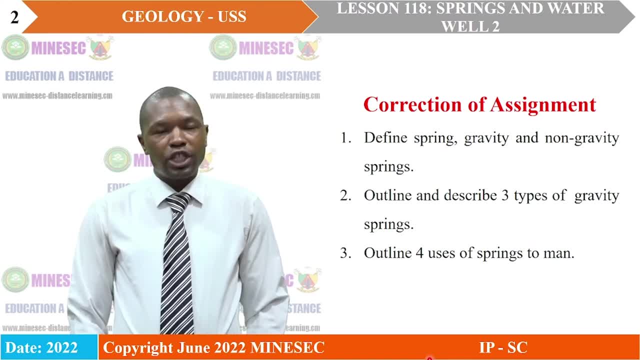 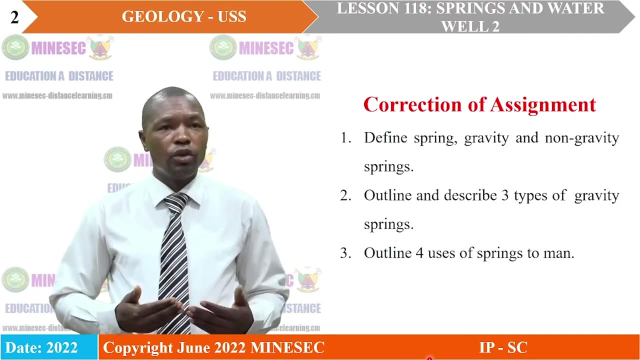 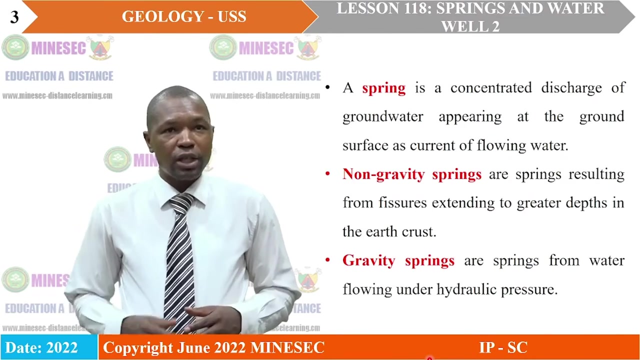 describe three types of gravity springs, Then align four uses of springs to mind. Four uses of springs to mind. These are AC-type equations and it involves that we express our know-how. So correct answer: A spring is a concentrated discharge of groundwater. 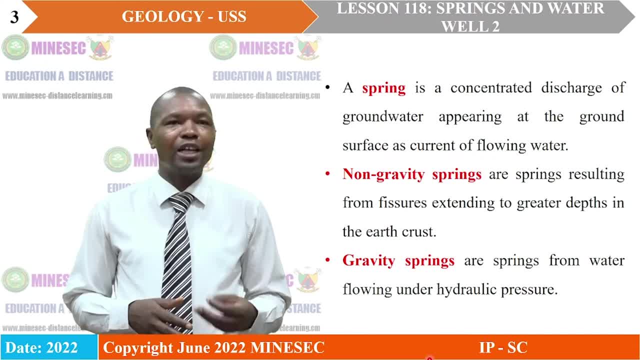 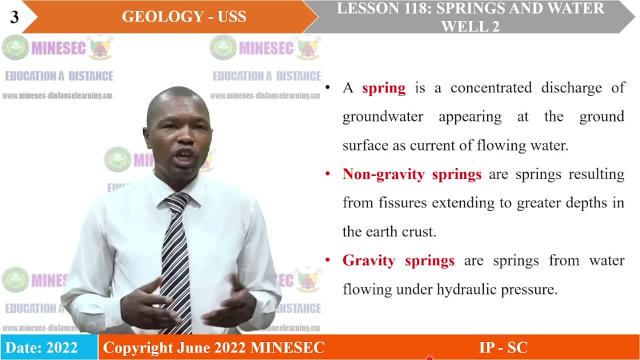 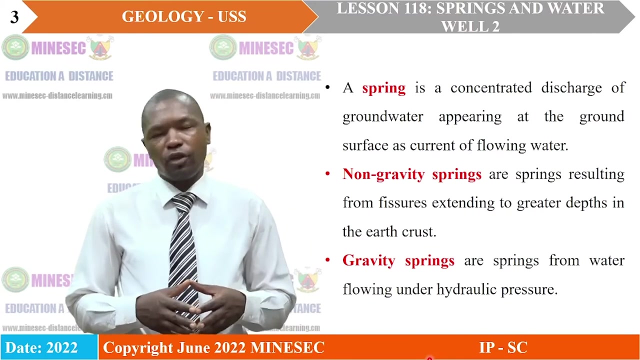 appearing at the ground surface as a current of flowing water. We equally said it is water on the surface when the water table is intercepted. Non-gravity springs are those springs resulting from fusions extending to greater depths in the earth's crust, meaning that they are springs. 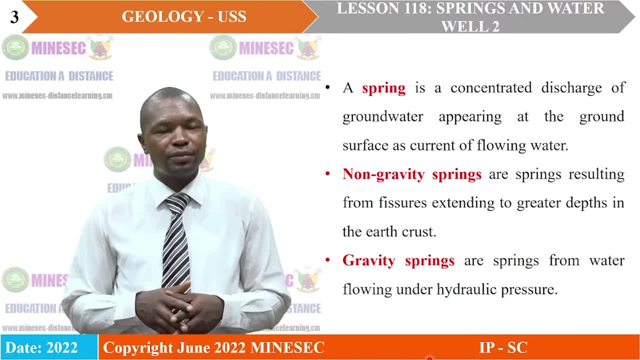 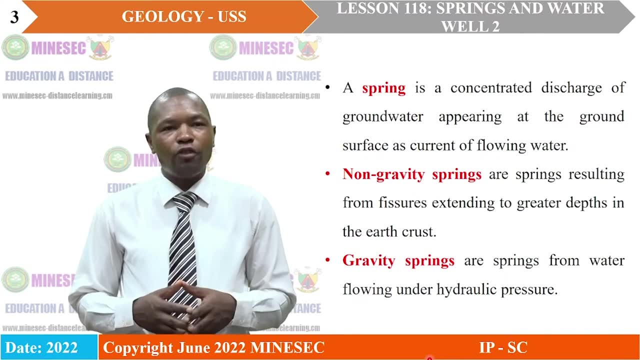 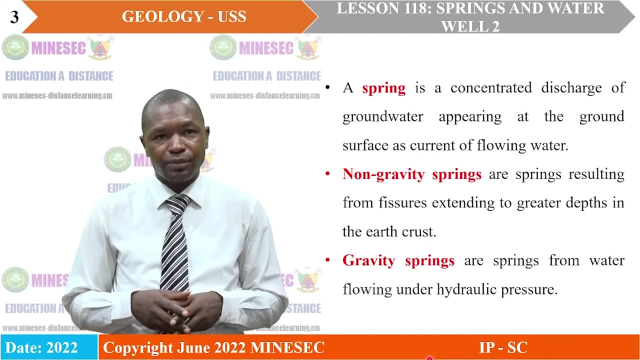 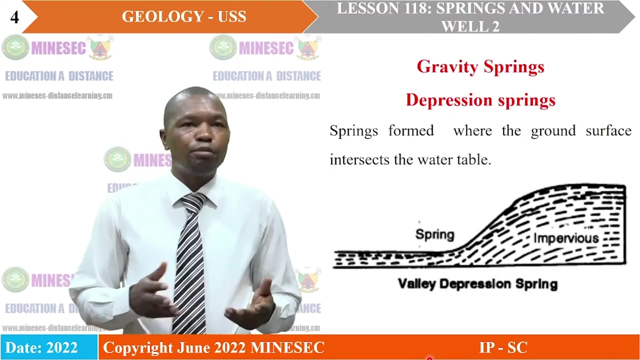 that are related to magmatic activities. Gravity springs are those springs that result from water flowing under the hydraulic pressure, better still, under the influence of gravity. That was part one of the question. Then part two: we are required to align three as well. 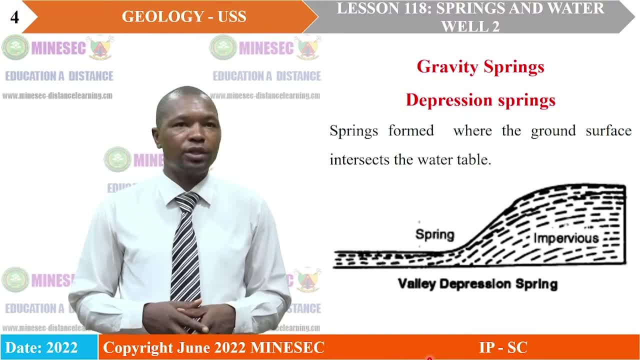 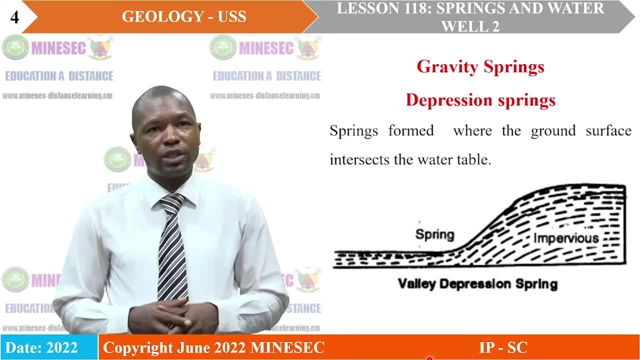 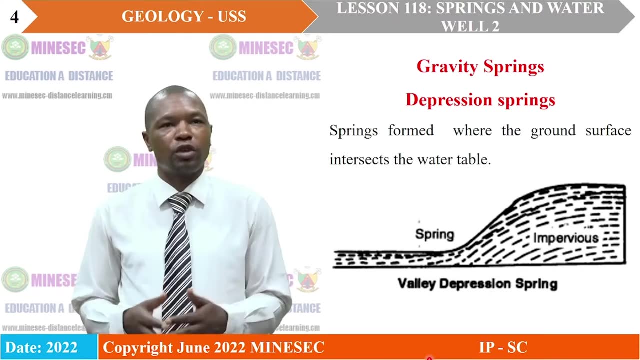 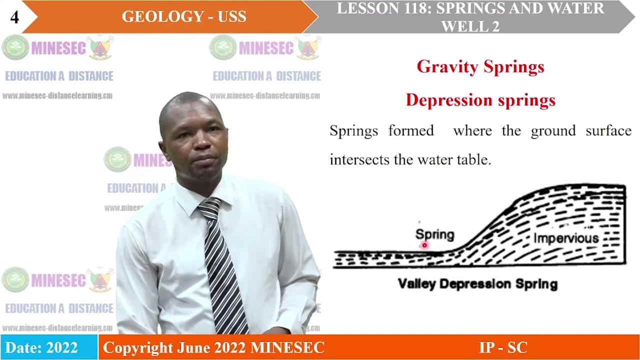 as describe three gravity springs. The three gravity springs will just be outlined and described in advance. The first is depression springs. These are springs formed where the ground surface intercepts the water table, As you can see illustrated in the diagram. Then we have contact or unconformity. 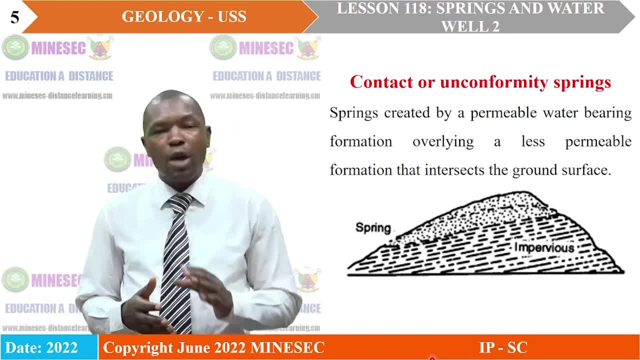 springs. These are springs created by a permeable water bearing formation Overlying a less-permeable formation of water. these springs lead us to the following: drilled, drilled. drilled- This injects water through the excess air intake. изEX, colors: This injects water through. 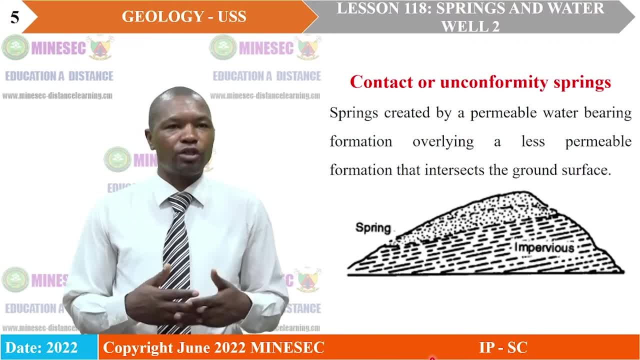 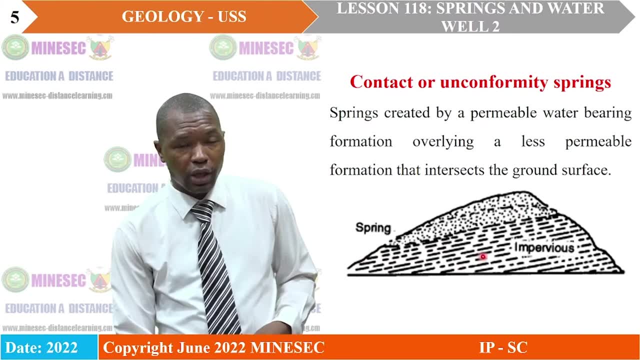 the excess air intake and Druck pressure. This inject. this injects 무엇en water production, create a density that intercepts the ground surface, as we can see in our illustrative diagram. you see here, this is the water table. this is a an impermeable layer. and then, above the water table, you also have another. 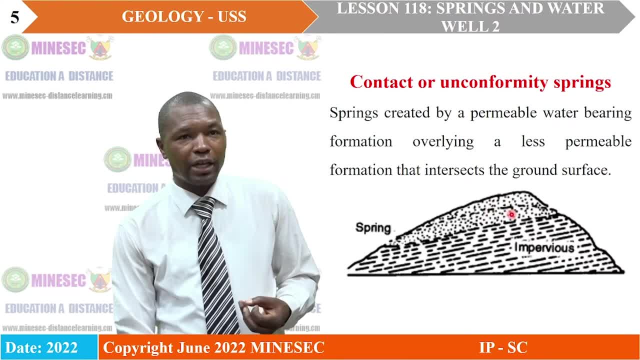 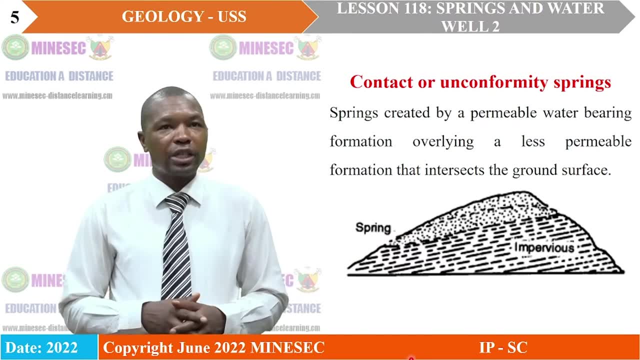 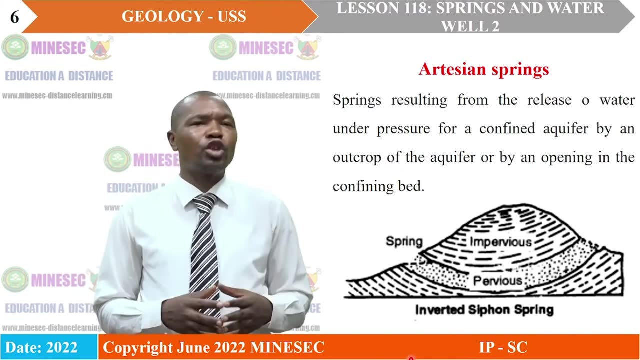 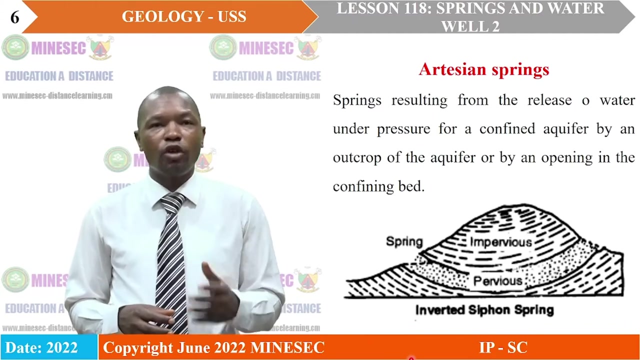 layer that should be a water bearing layer so they intercept the surface and flow. we call it contact or unconformity spring, now artesian wells or artesian springs. these are springs resulting from the release of water under pressure for a confined or from a confined aquifer by an outcrop. 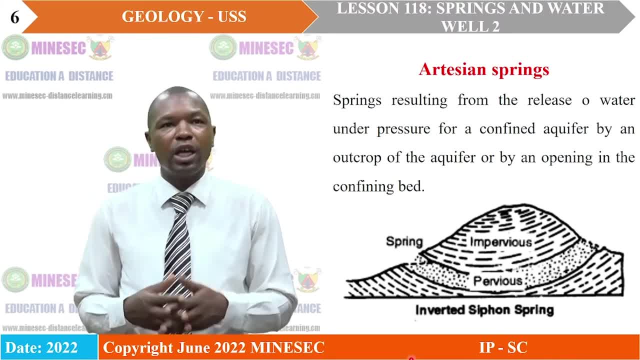 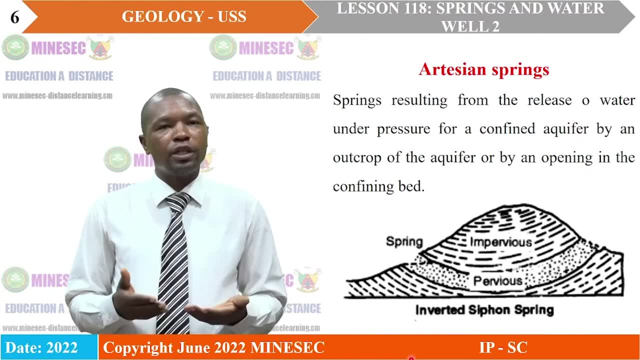 of the aquifer or by an opening in the confining bed. so there are different dimensions. you can tackle it it it could be the fact that that the confined aquifer is intercepted so that water can flow from it on the surface, or an unconfined aquifer is intercepted so that water flows on the surface on its own. 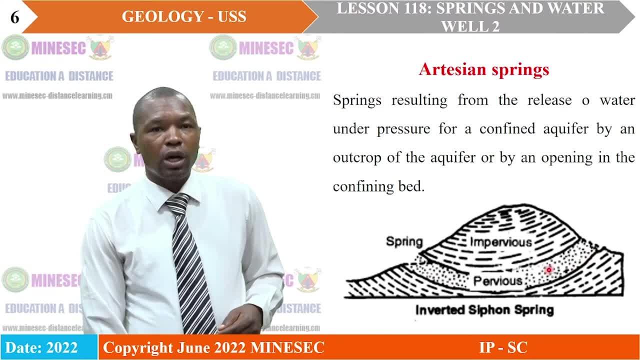 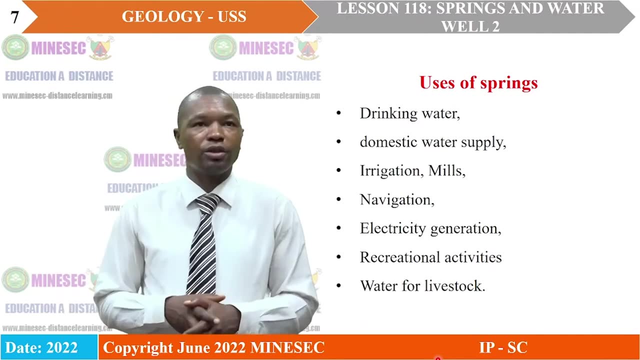 As you can see it illustrated in the diagram, This is a permeable layer. this is impermeable. this is impermeable. So here you will find there is interception, and then water flows on the surface. That gives birth to artesian worlds. 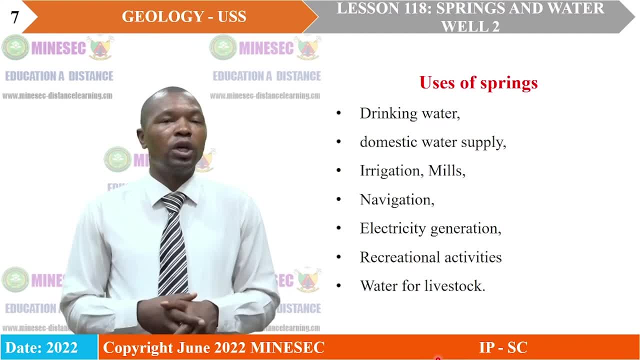 The third part of the equation requires that we should discuss the benefits of springs. to mine We are asked only for four, but we have an alignment of meaning. We have. it could be used for drinking water. It could be used for drinking water. 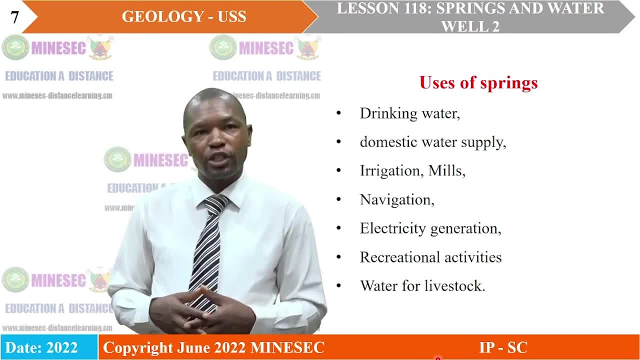 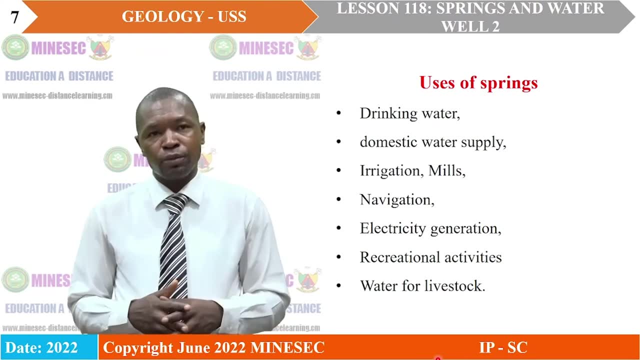 It could be used for drinking water. It could be used for domestic water supply. Springs could be used for irrigation and for mills. It could also be used for navigation. Springs can be used for electricity generation. They can also be used for recreational activities as well as springs can be used or conserved. 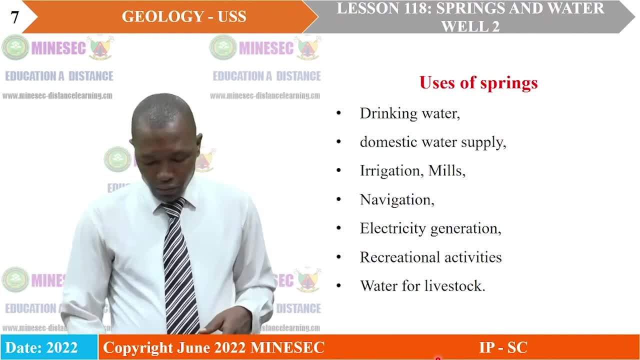 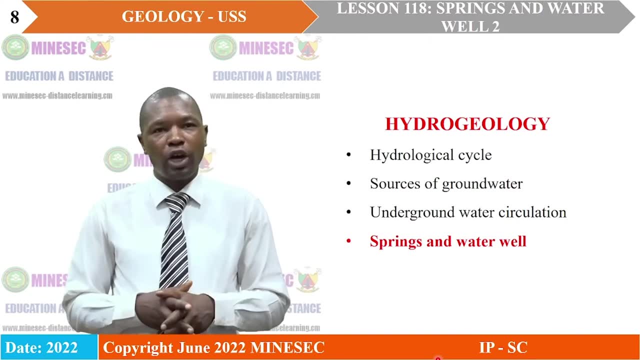 as water for livestock. Okay, We continue with our topic of hydrogeology. Well, we already saw hydrological cycle. We saw sources of groundwater. We equally looked at underground water circulation. We concentrate on springs and water wells. During our last lesson we had treated a portion of water wells. 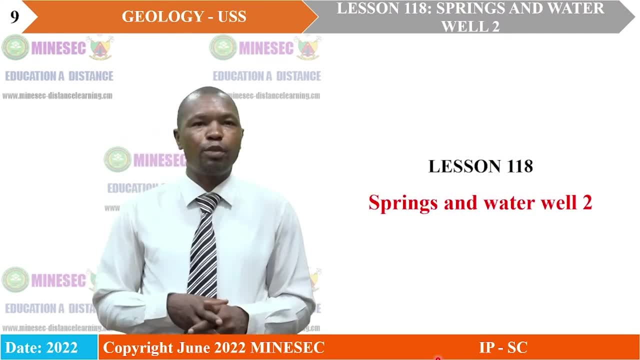 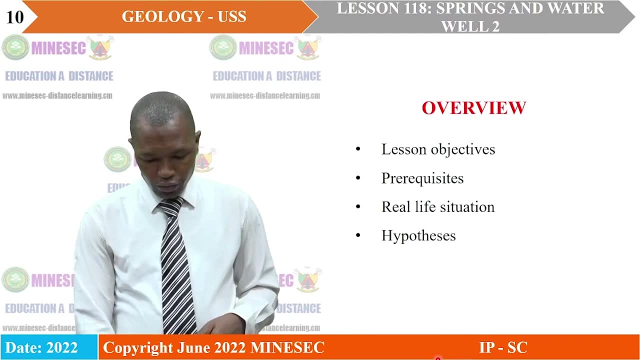 So our lesson 118 is titled Springs and Water Wells 2. Springs and Water Wells- 2. Now you will realize that springs and water wells are two different things. Now you will realize that springs and water wells are two different things. You will realize that in order to grasp the concept of springs and water wells, it will 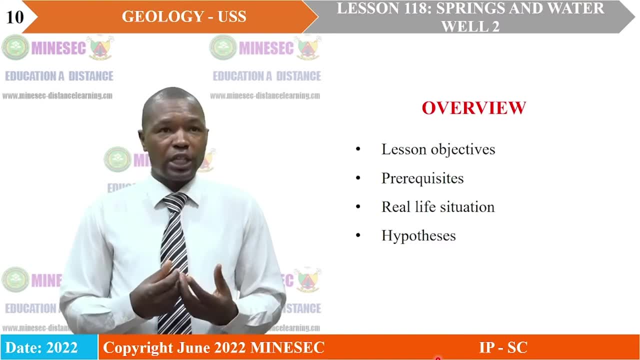 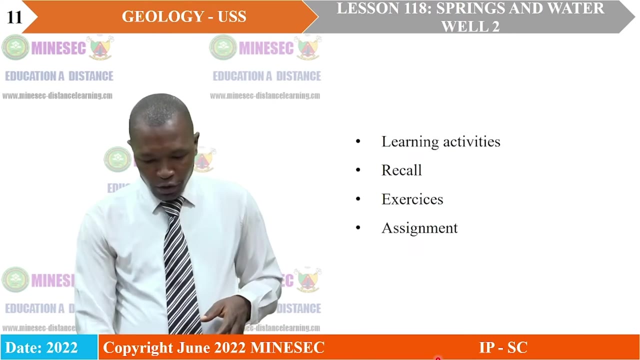 be important to have some objectives and come up with some prior information that is more related to hydrogeology. Then we will have a real life situation and come up with some hypothesis. Then we will go through some learning activities that will help us to exploit the content of. 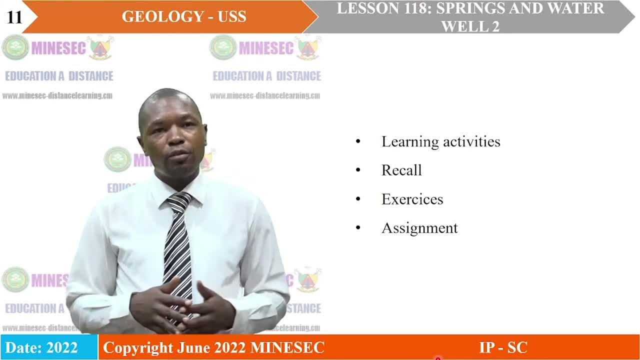 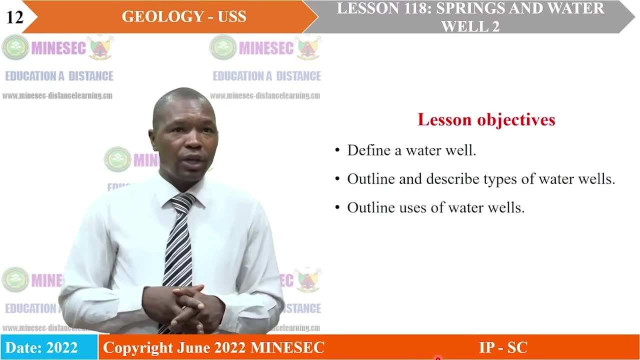 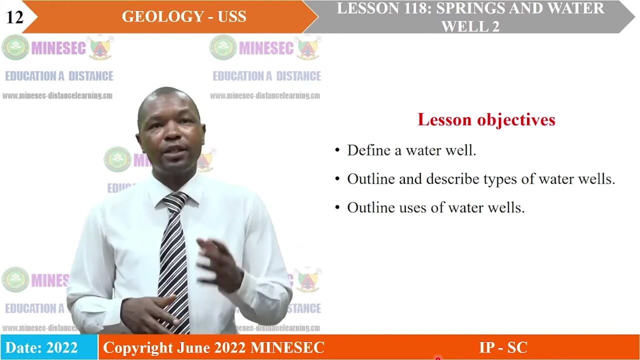 our lesson. then we will have a recall, have some application exercises and end the lesson with an assignment. today our learning objectives will be to define a water well- there is a specification water well, not just a well water well. then we will align and describe heights of water wells. then we will also be able to come out with the uses of. 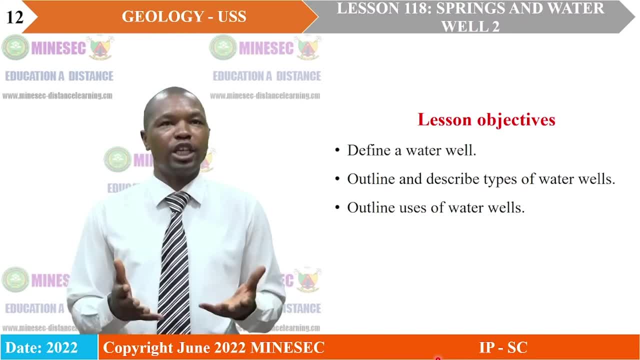 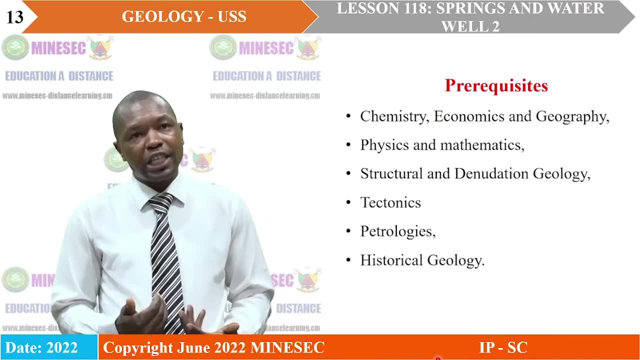 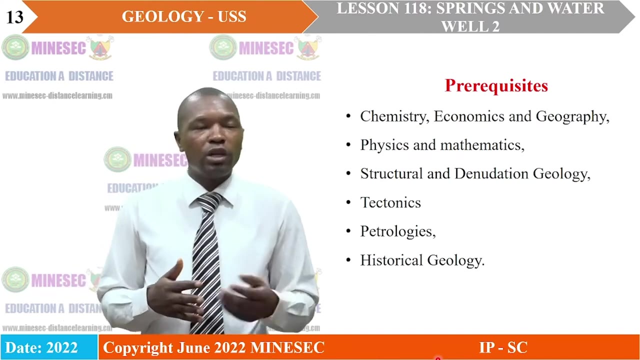 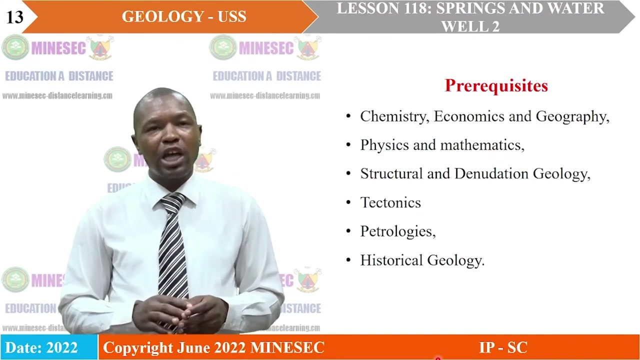 water wells to man. remember that we are treating economic geology. now, knowledge that is necessary for us to have a better understanding of water, water wells, will come from a knowledge of chemistry, economics and geography. particularly in geography we look at climatology. those are the different areas, or different. 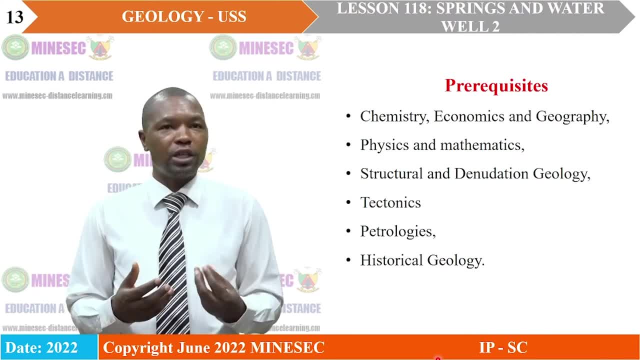 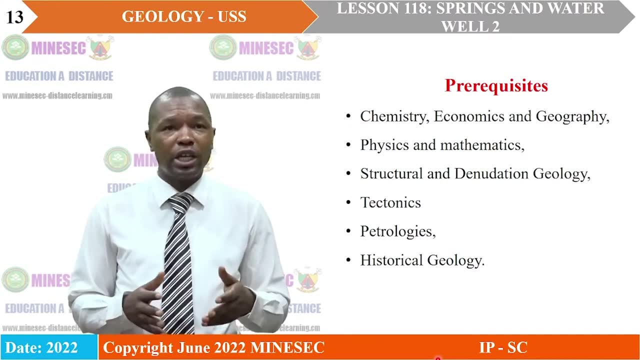 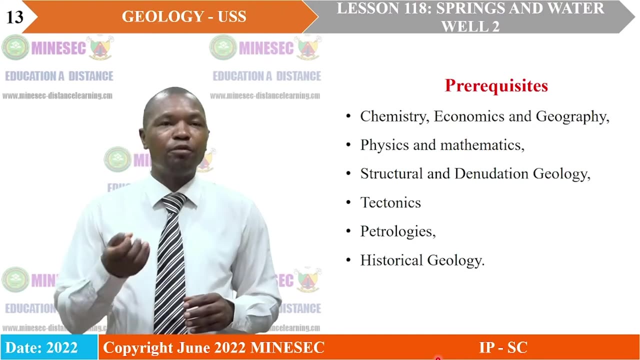 aspects through which you know water or material water is gotten, which is the primary source of groundwater or the primary source of water in the water table, then those underground water reservoirs are exploited, and they can be exploited using the knowledge in physics and the knowledge in mathematics. 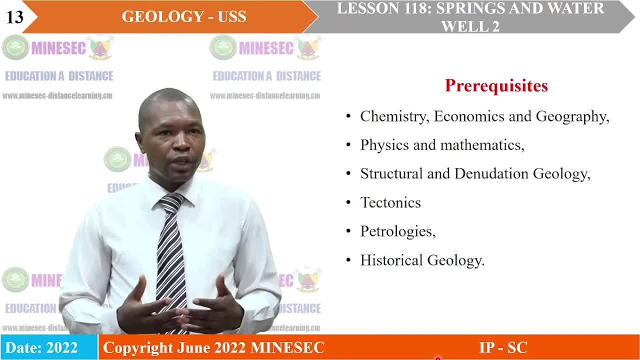 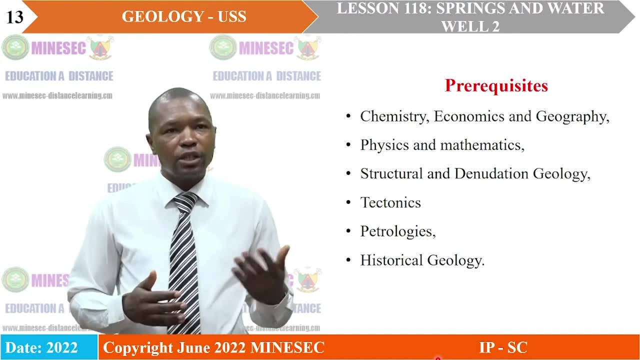 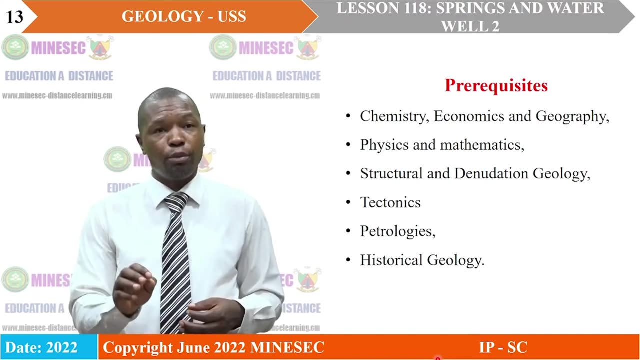 also, water has to move through the ground, so the knowledge of structural and denudational geology is vital. again, there are forces that have to drive the movement of water, so knowledge on tectonics is very important. water cannot move in space alone. water has to move. 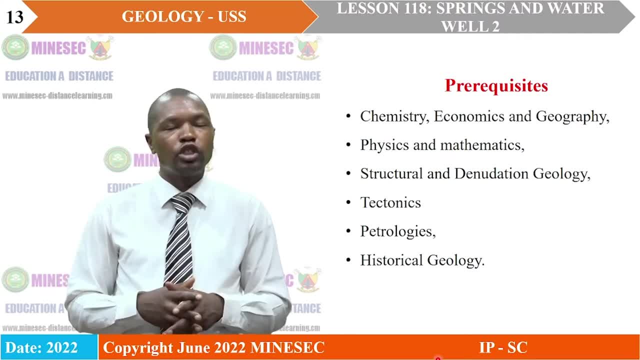 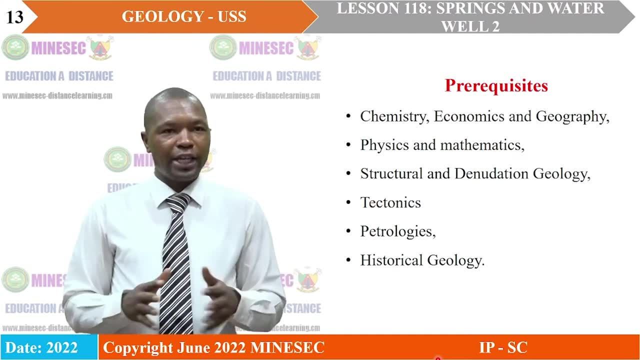 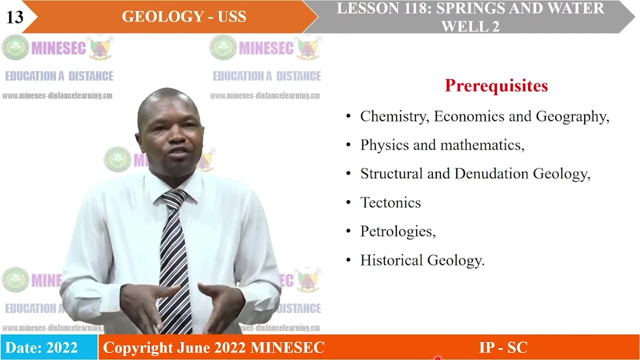 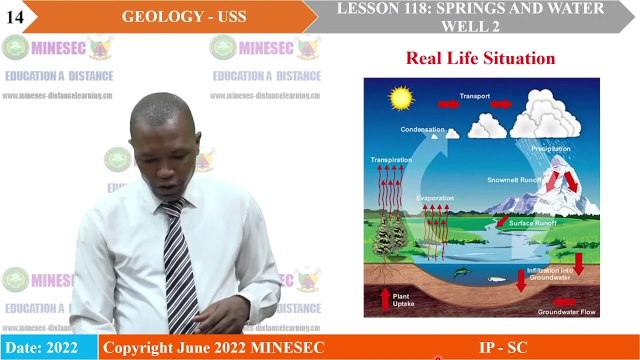 through the different rock types. so knowledge of the different petrological types, that is, igneous, sedimentary and mermorphic petrologies, are vital. water has, to you know, coordinate itself within strata, so the knowledge on stratigraphy, as well as paleontology, is vital here. this way, 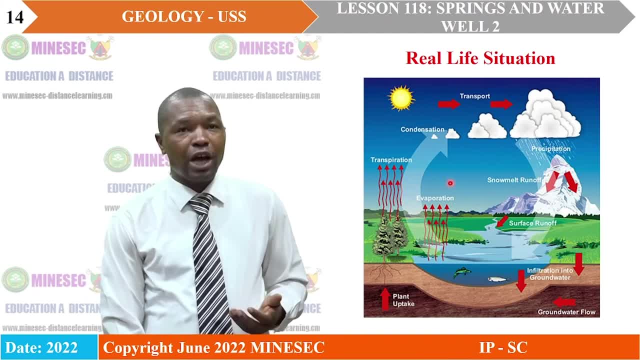 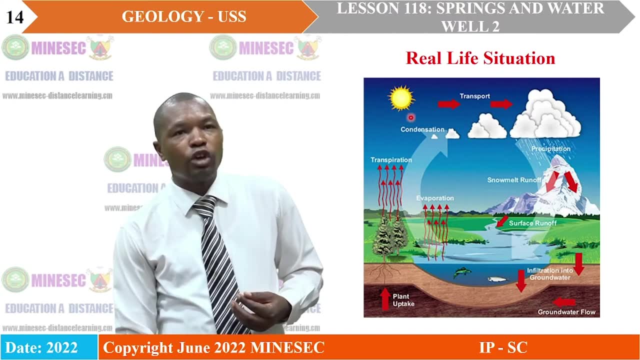 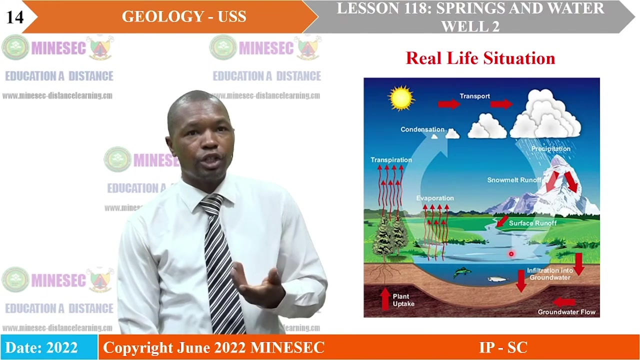 look at this photograph to have an understanding and then develop our real life situation. Now you realize that there is a relationship between the sun, the clouds, that is, water above the surface, and water on the surface through different water bodies like running water or rivers or oceans. 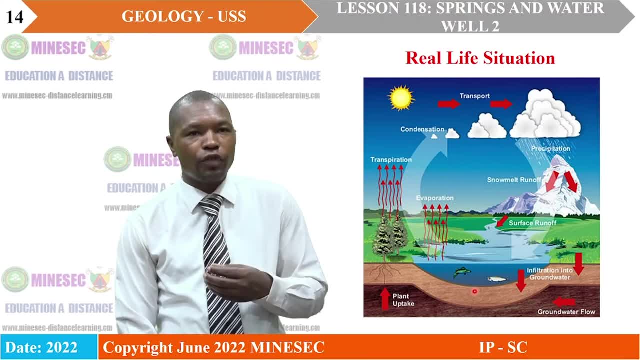 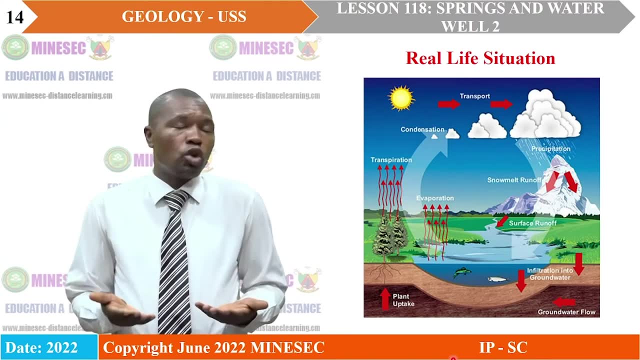 And then that relationship doesn't end only at the surface, It also goes beneath the ground. So we are saying that from our illustrative diagram there is a relationship between water above the surface, water on the surface, and water beneath the surface. 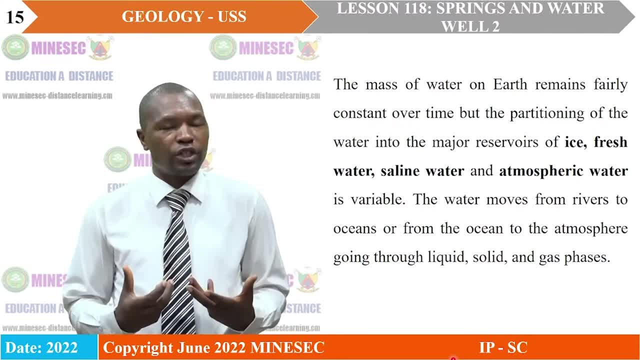 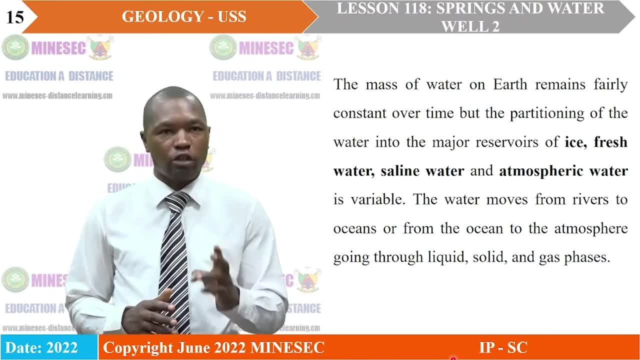 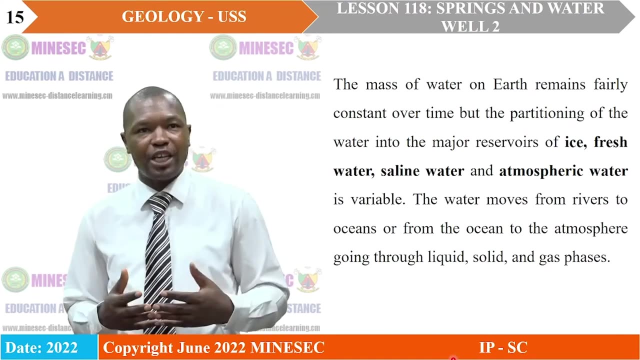 So it helps us to be able to push this concept, or to develop this concept, that the mass of water on the earth remains fairly constant over time, But the partitioning of the water into the major reservoirs of ice, fresh water, saline water and atmospheric water is varying or is variable. 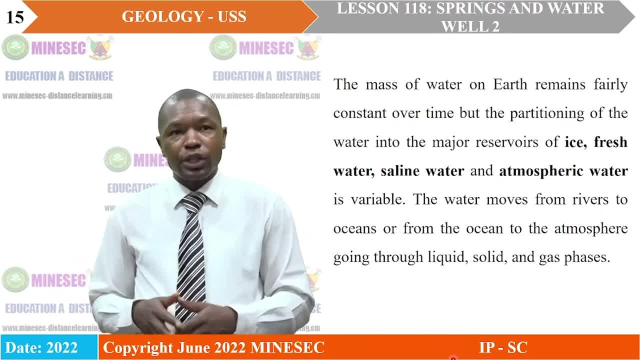 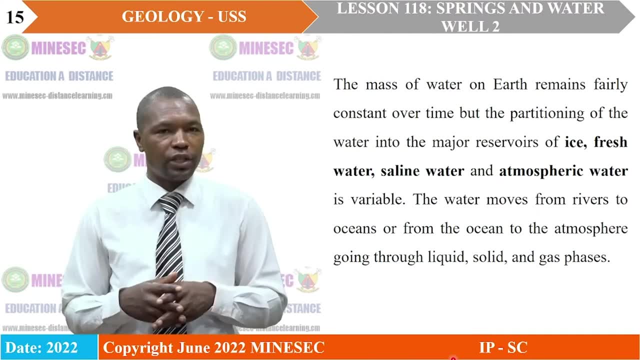 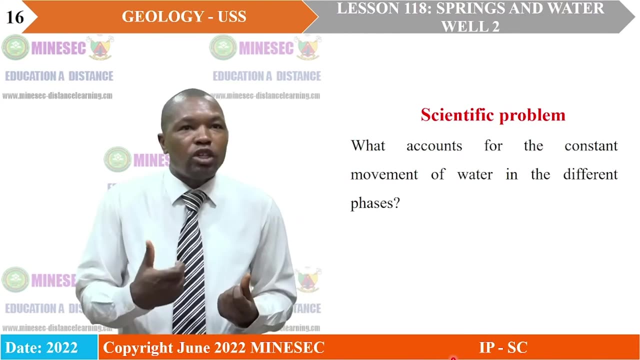 Now the water moves. It moves from rivers to oceans or from the ocean to the atmosphere, going through liquid, solid and gaseous phases. The problem is this: that you know what can be or what will account. what is the mechanism for this constant movement of water in the different phases? 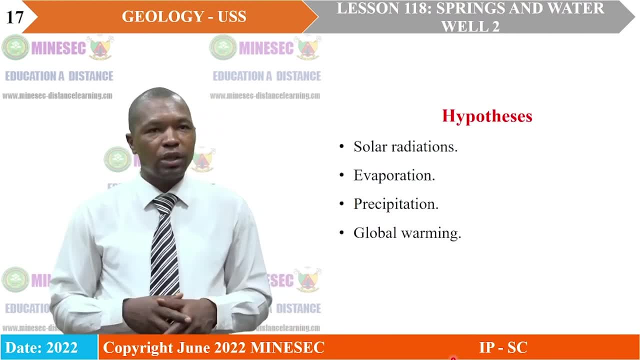 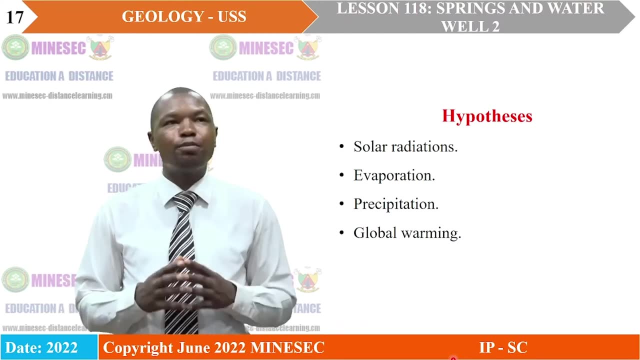 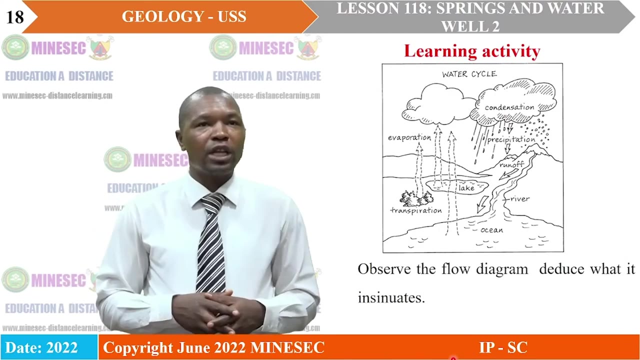 Is it based on solar radiation? Is it based on evaporation? Is it based on precipitation? Is it based on global warming? As we exploit the content of our lesson, we are going to discover which of these hypotheses is correct. Now, in our learning activity, we get again to this illustrative diagram. 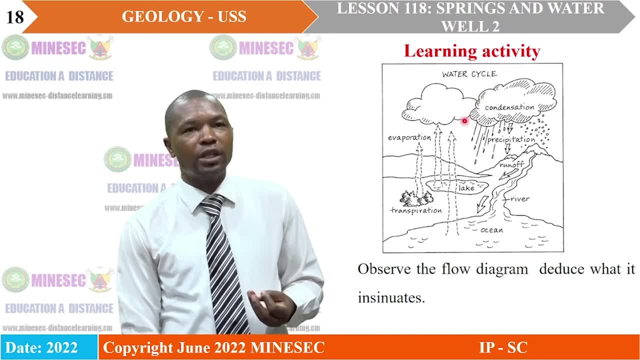 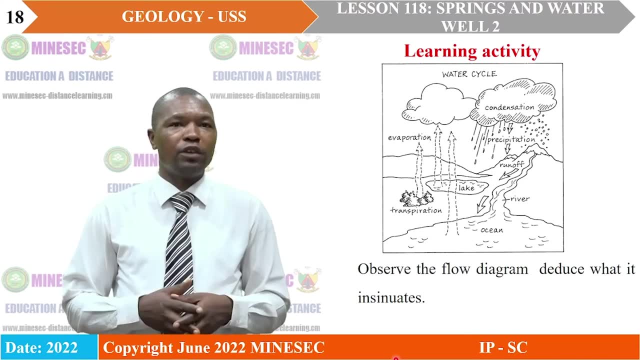 where you have the relationship, as in the water table. Remember that the water table has a relationship with water above the surface, with water on the surface and water beneath the surface. Remember that our concentration now is water beneath the surface. How is it? 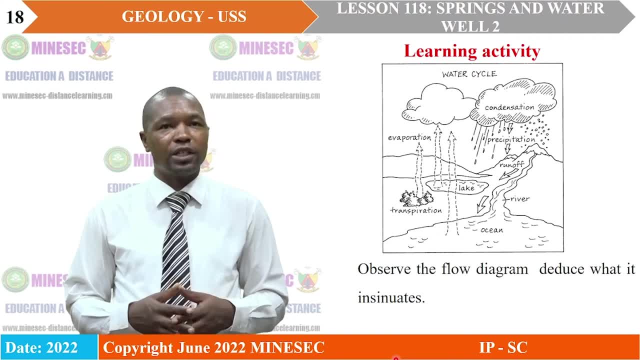 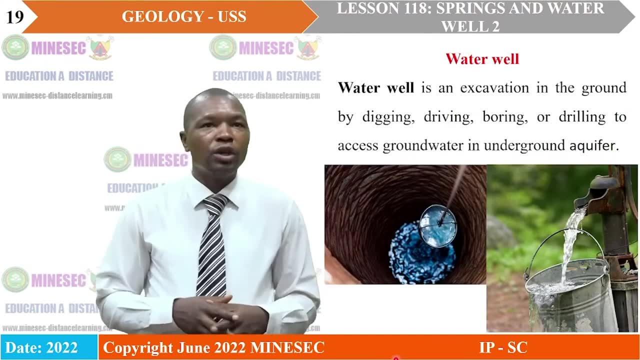 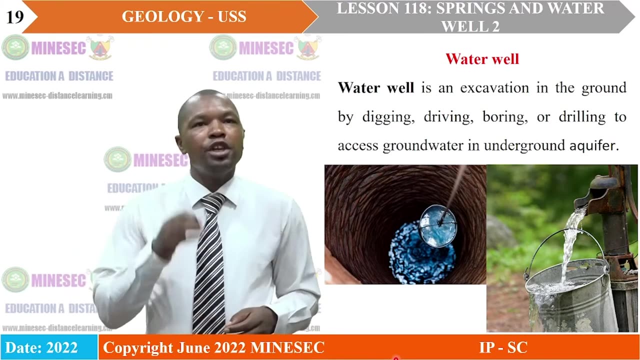 How is the water stored? We already evoked during the first lesson that water is stored through springs and water wells. Now we already saw springs. We're going to continue with water wells Now. a water well is an excavation in the ground. 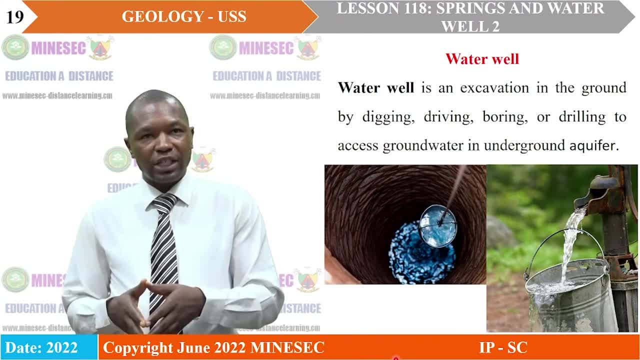 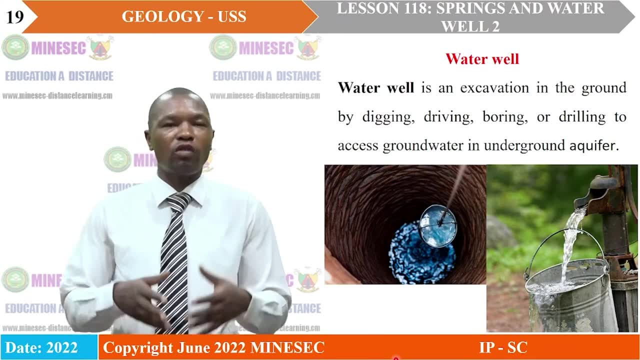 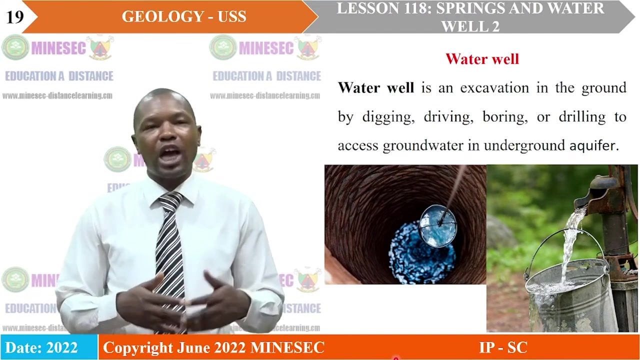 by digging, driving, boring or drilling to access groundwater. to access groundwater. The reason for the digging, for the driving, for the boring, for the drilling is such that groundwater is intercepted. That is what is generally referred to as boreholes. 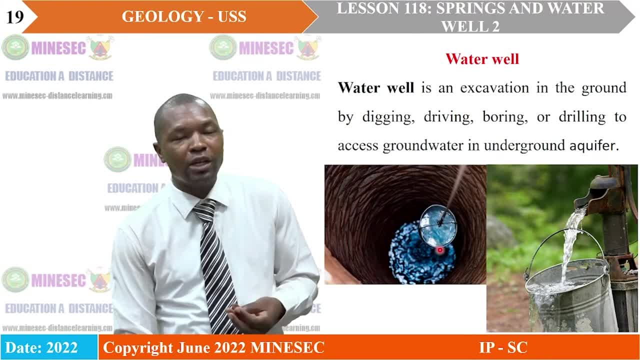 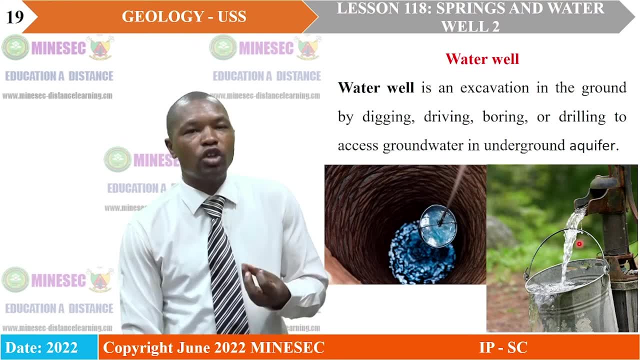 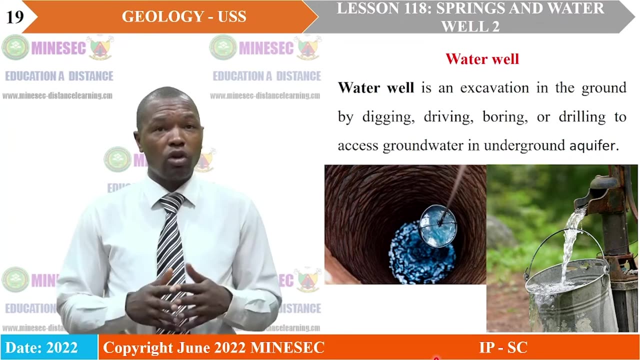 Look at here. This is a borehole from which water can be gotten, And then you also have now a borehole where water is already on the, where the water families are being used. So a well is not, or a water well is not, or drilled to obtain water. 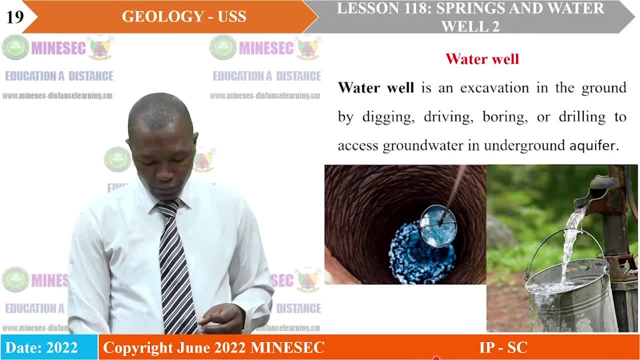 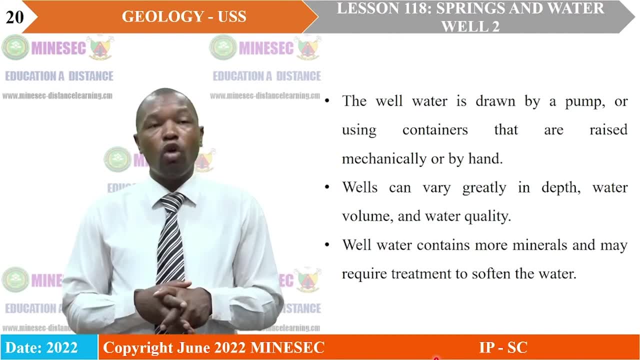 that you get from the groundwater. Now the well water is drawn by a pump or using containers that are raised mechanically or by hand. You know the most common. you have the hand system and the pulley system, And then you have the slide system. 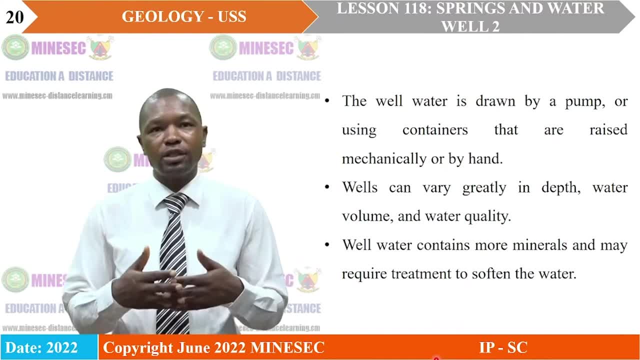 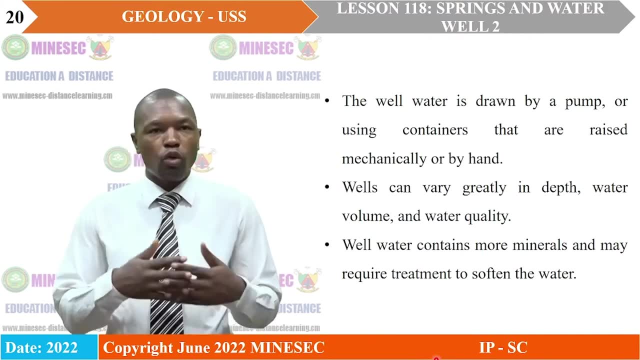 And you have the hand system. Wells can vary greatly in depth, They can vary in water volume and they can vary in water quality. Water well contains more minerals and may require treatment to soften the water. We know that there is a difference between hard water and soft water. 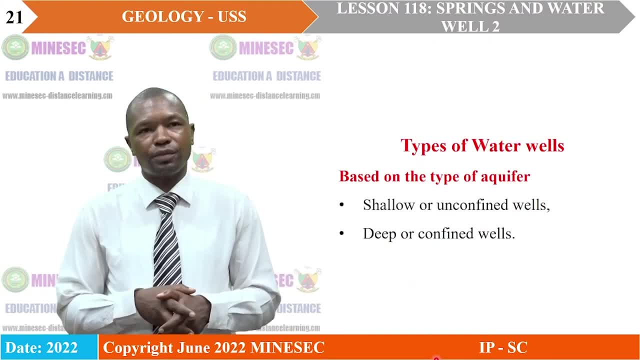 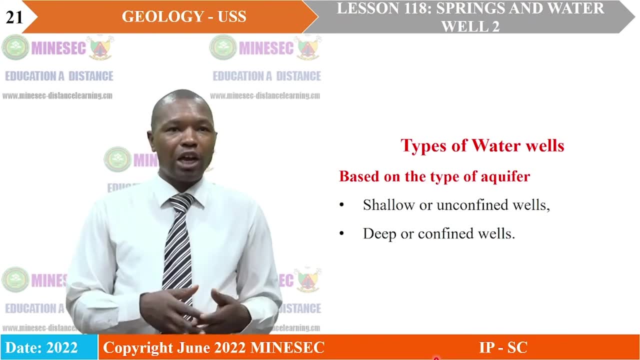 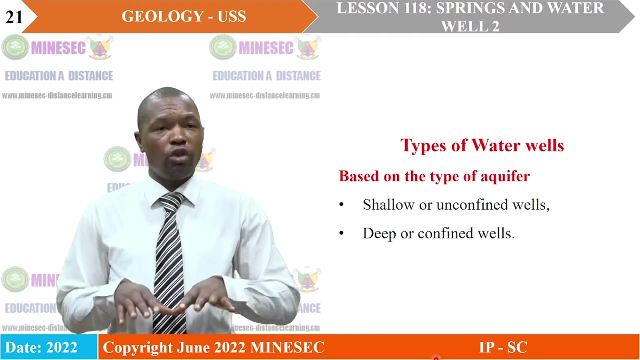 Now we go to types of water wells. Now, based on the type of aquifer in which the well is drilled, we can have shallow or underground wells. We can also have deep or confined wells. So in reality we have two groups of wells based on the type of aquifer. 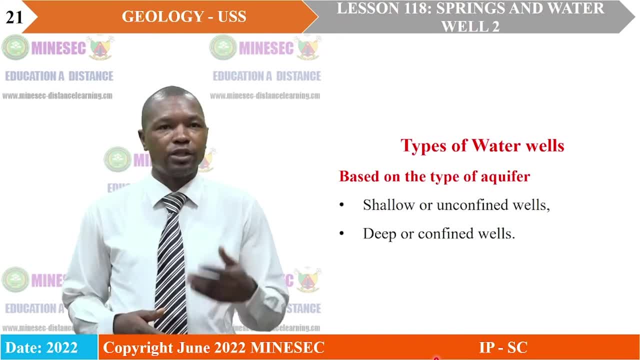 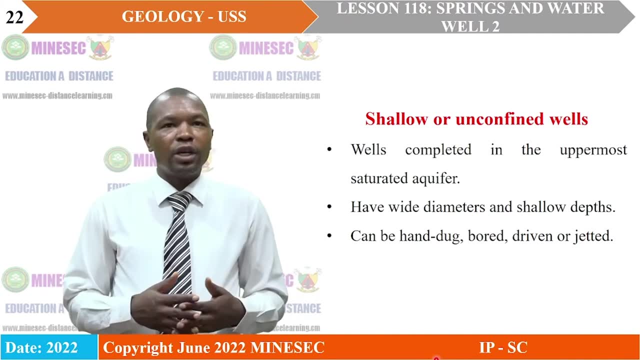 That is shallow and deep, or on confined and confined wells. So shallow or on confined wells, These are wells That are completed in the uppermost saturated aquifer. So a shallow well is a well that is completed in the uppermost saturated aquifer. 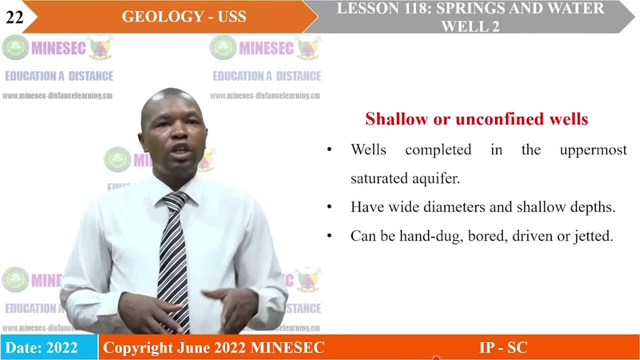 It means that the aquifers are not deep, Then they have a wide diameter, Or they have wide diameters and shallow depths. They can be hand dug, Meaning that the digging can be done manually, Mechanically, by Locally, by man. 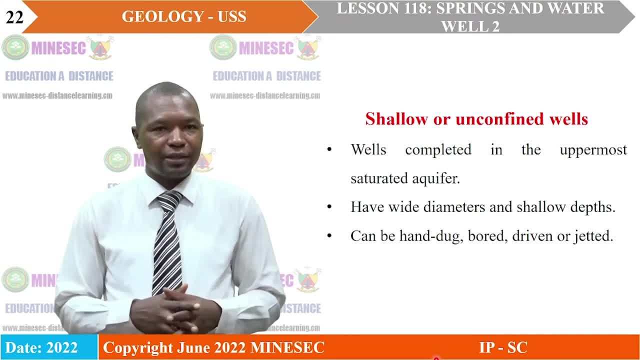 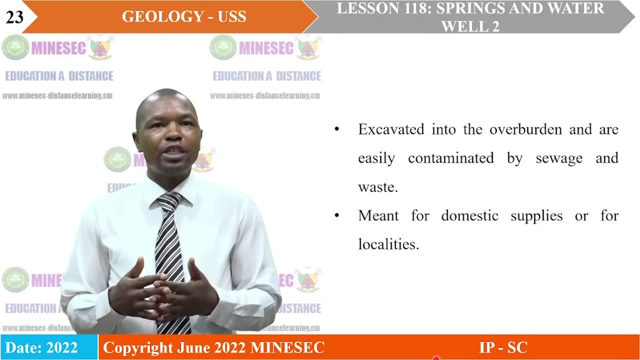 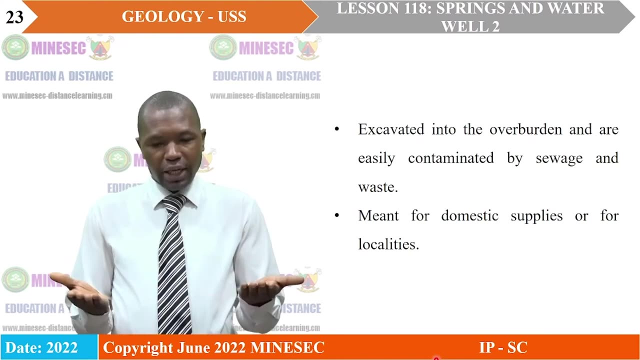 Or they can be bought. They can also be driven, Or they can be jetted. These kinds of wells are excavated into their overburdened and are easily contaminated by sewage and waste, Since there are shallow depths. what happens is that if there is a contaminant, 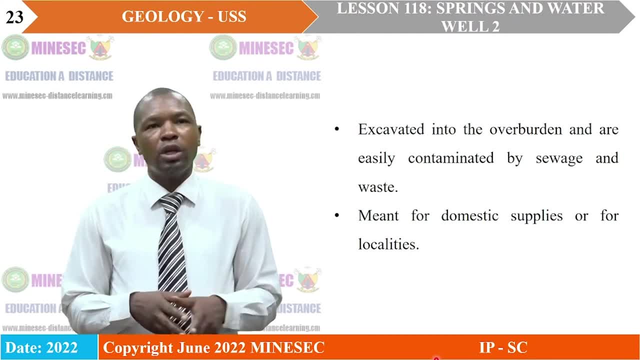 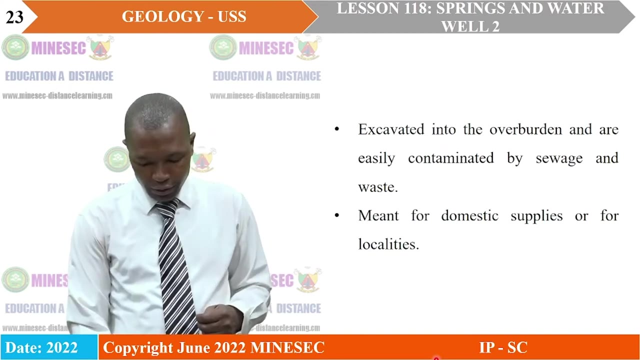 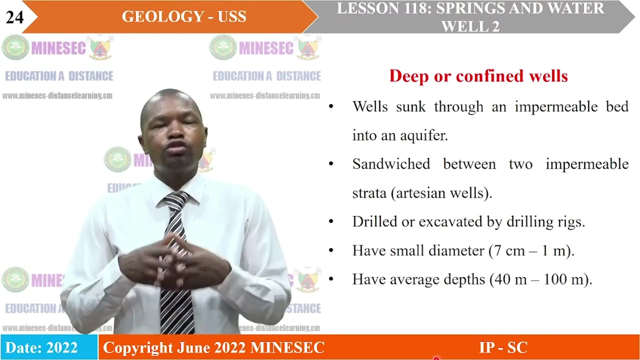 it will quickly get into the groundwater soils. They are meant for domestic supplies Or for localities. You could have a community project for boreholes, like what mostly happens around the country Cameroon. They have deep or confined wells. They are wells sunk through an impenetrable bed, into an aquifer. 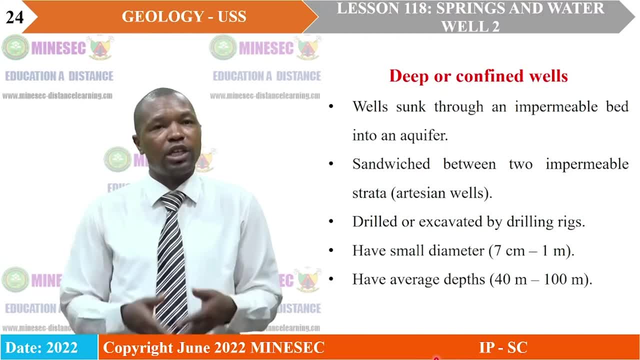 Meaning you have to. they are not like shallow wells where you just get straight to the aquifer. You have to go through an apricot before you arrive. You have to go through an apricot before you arrive The aquifer. They are sandwiched between two impenetrable strata or beds. 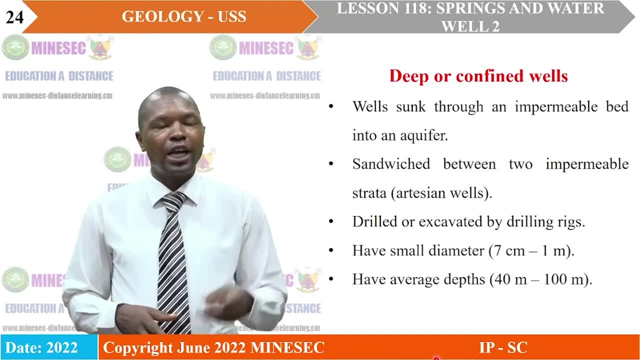 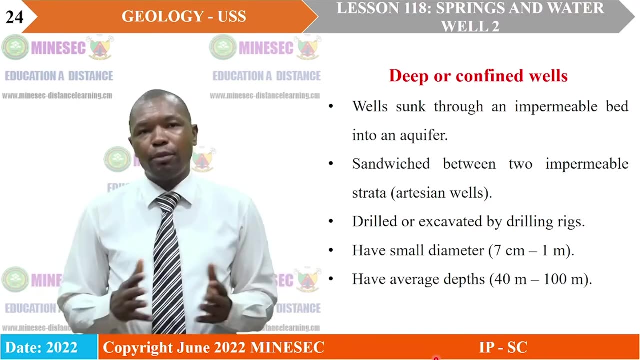 That is the reason why we call them artesian wells, And they are drilled or excavated by drilling bridges because, or rigs because they have to go deep. Then they have small diameter of between 7 cm to 1 m. That is to maintain stability, in order not to create danger. 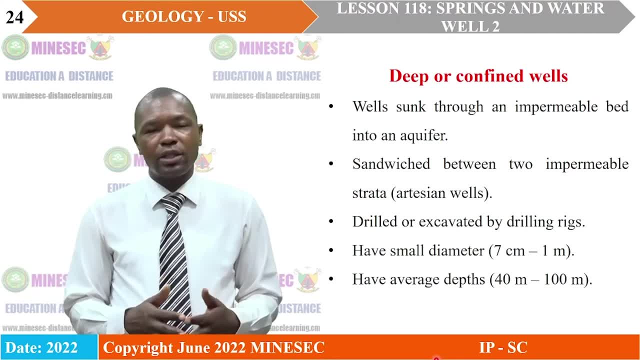 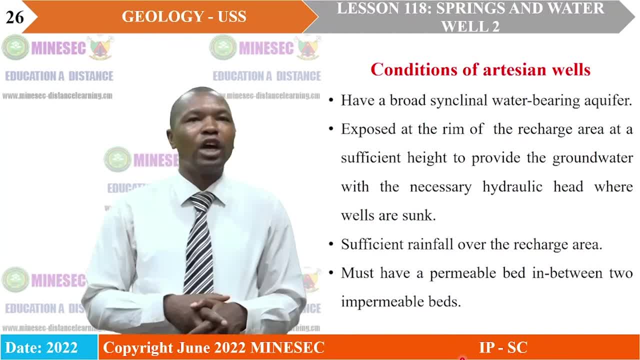 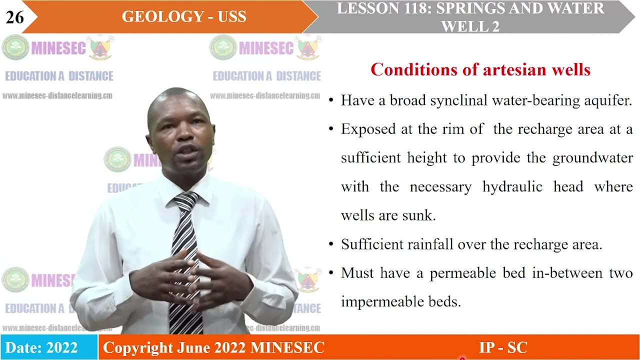 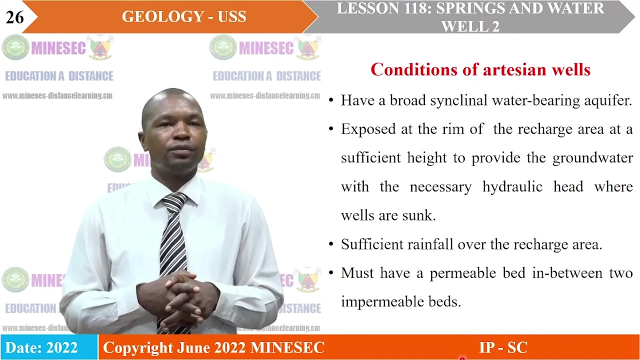 its own force. now you have the conditions of artesian wells. for any well to be to be artesian, it must fulfill those conditions. one, that the world must have a broad cylindrical water bearing aquifer, have a broad cylindrical water bearing aquifer. secondly, it must be exposed. 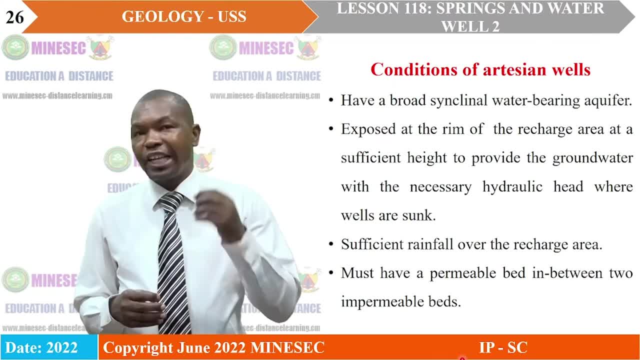 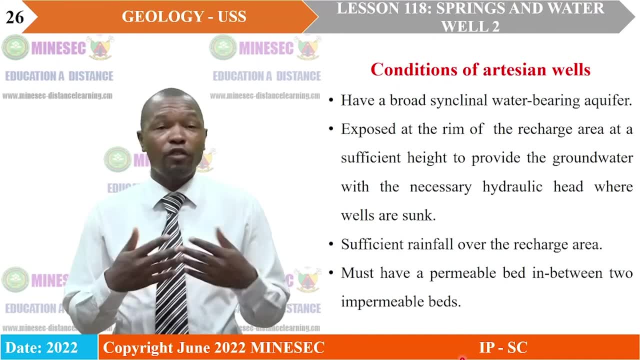 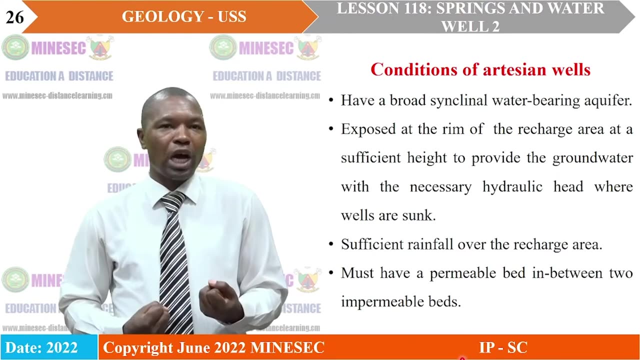 at the rim of the recharge area at a sufficient height to provide the groundwater with the necessity, or with the necessary hydraulic earth where wells are sunk. this way it will be able to give the world capacity to order water, the capacity to flow by itself. then such a world 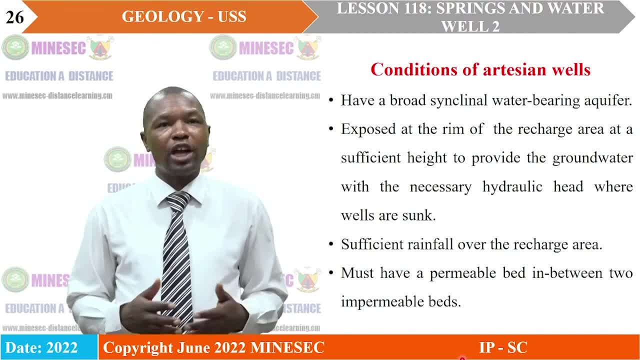 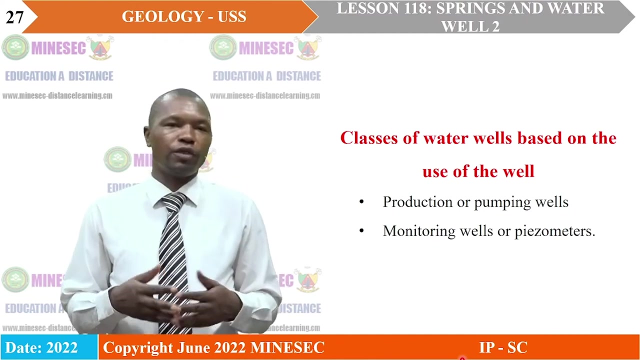 should have sufficient rainfall or such an area should have a sufficient rainfall in order to boost the recharge of water in the world then they must have a permeable bed in between two impermeable beds meaning there should be a confining surface � � m of water well 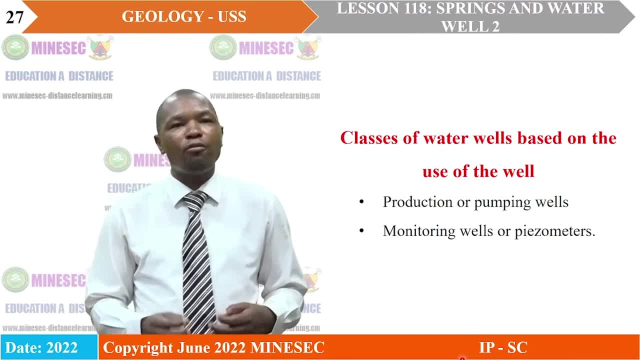 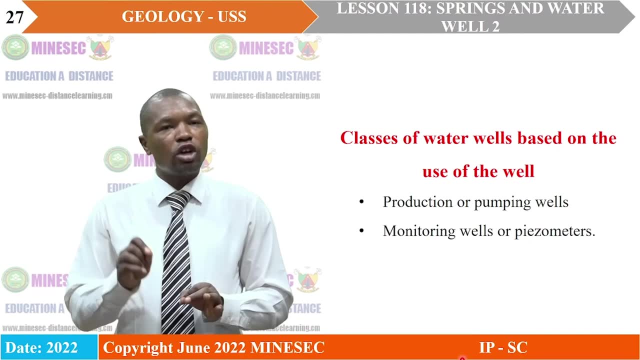 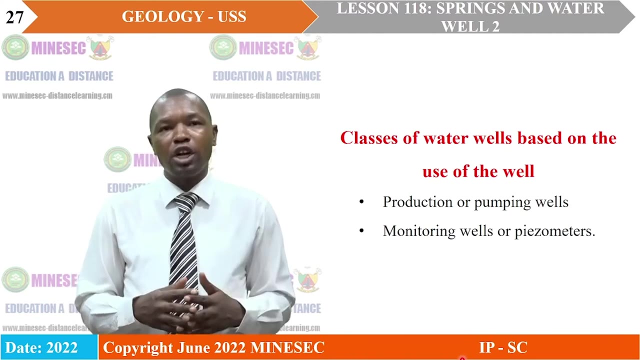 various water modes are commonly involved in the glass we have to consider we often think of. We have productive or pumping wells and we also have monitoring wells or piezometric or piezometers Based on the use of the well. we have two productive or pumping wells and then we have monitoring wells or piezometers. 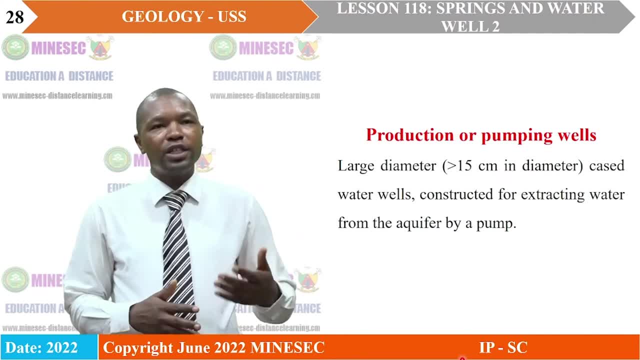 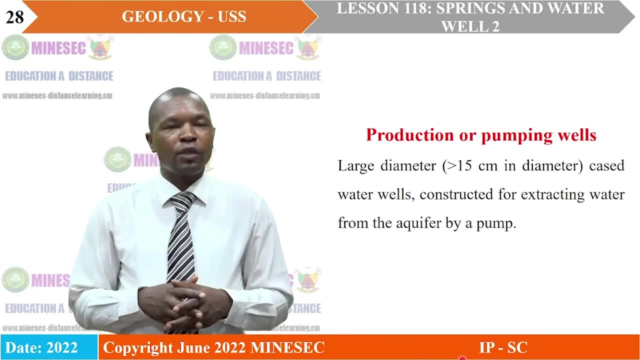 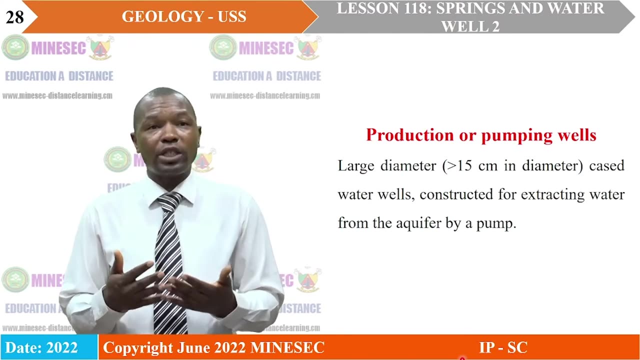 Productive or pumping wells. These are wells with a large diameter, of greater than 15 centimeters in diameter, And it is the case where water or the kind of water wells where the borehole is constructed for extracting water from the aquifer by a pump. 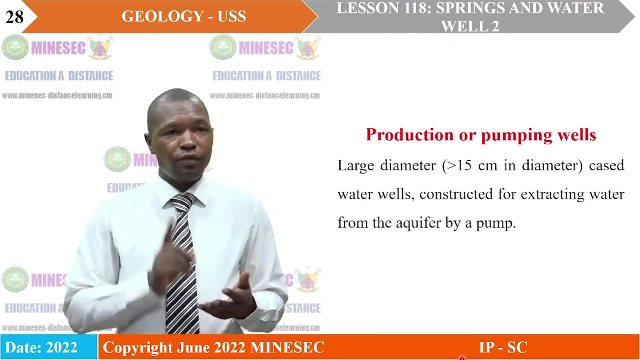 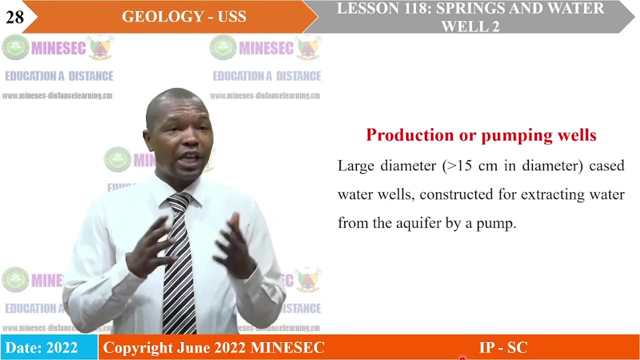 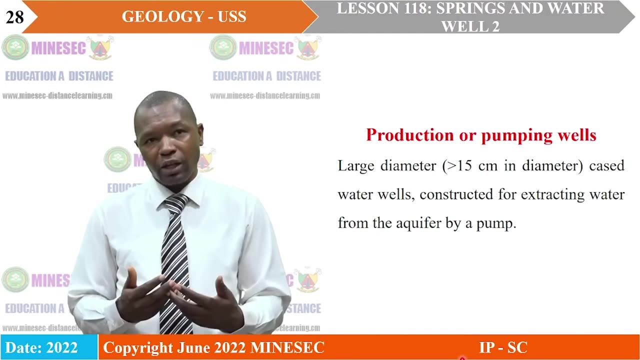 So in productive wells, first characteristic is that they have a large diameter Cased- okay, they are large diameter water wells And they are constructed for extracting water from the aquifer by a pump, You can call them. that is the reason why another name for productive wells is pumping wells. 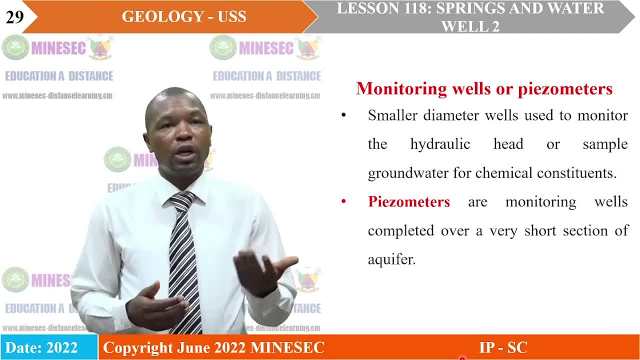 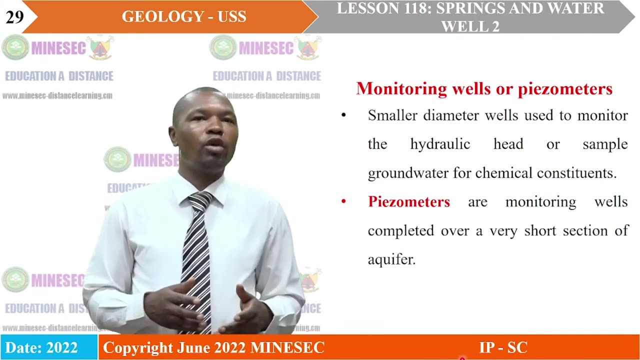 Now we have monitoring wells, Or better, if we have to reflect again on pumping wells, Those. these wells should be most likely related to what Shallow depth wells where you know water is gotten for domestic use. Then we have monitoring wells or piezometers. 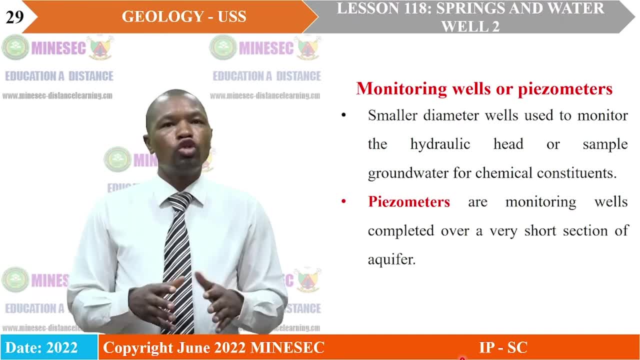 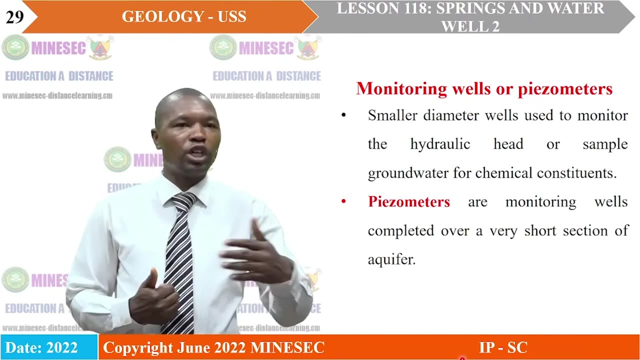 They are small diameter wells used to monitor the hydraulic head or sample water table or groundwater for chemical constituents. These wells could also be called research wells. They are used for monitoring, for research, for scientific research, For scientific programs that have to do with groundwater. 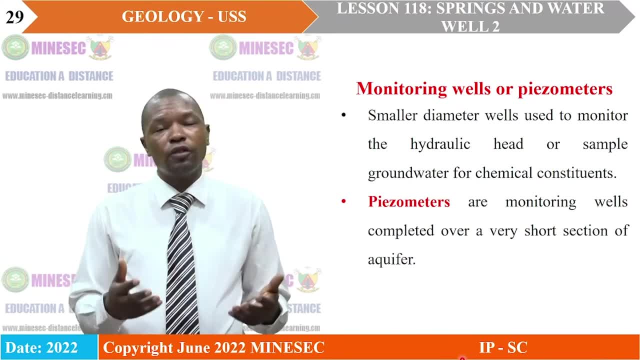 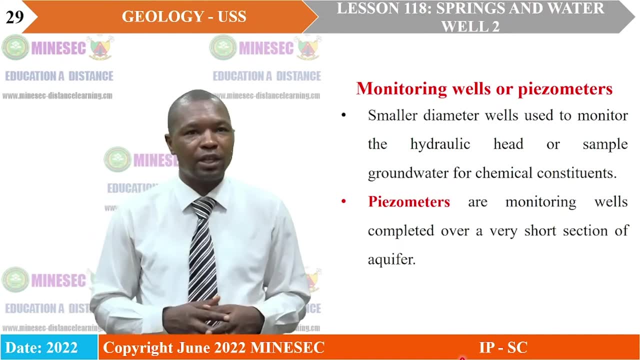 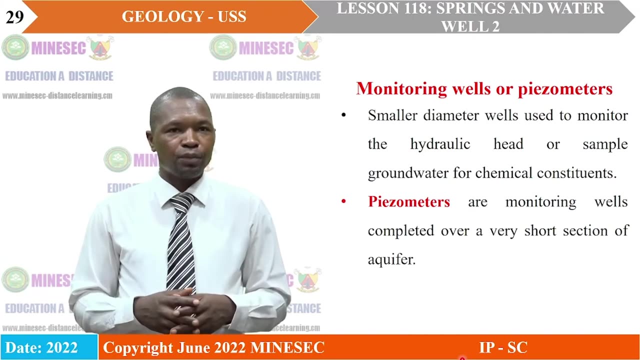 We also have it that they are used to monitor the chemical components or constituents of water. Then piezometers are monitoring wells completed over a very short section of aquifer. They are monitoring wells that are completed over a very short section of aquifer. 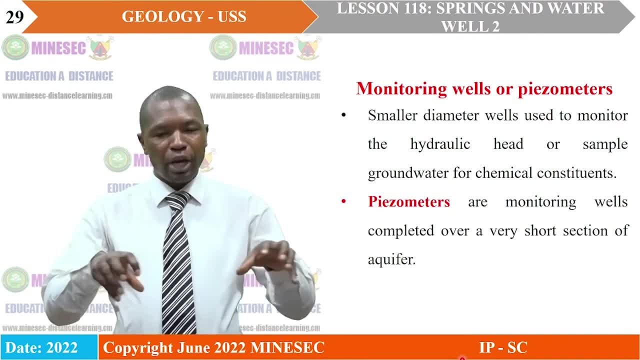 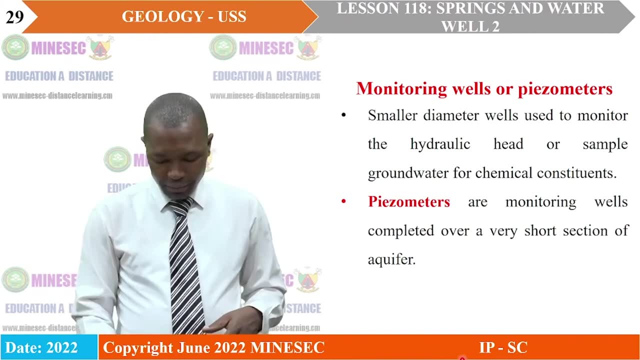 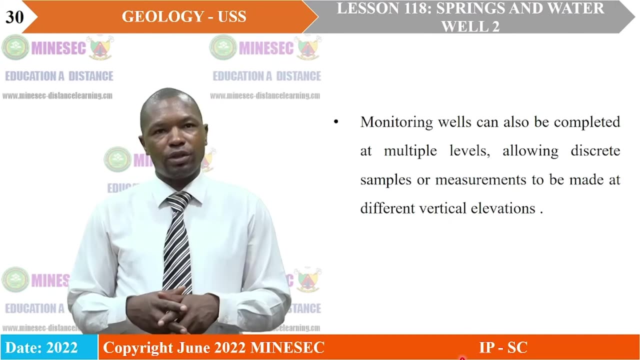 Meaning that there are. you know there are many of them within the same vicinity Purposely for monitoring. That is why we call them piezometers. Monitoring wells can also be completed at multiple levels, Allying discrete samples, or, you know, measurements to be made at different vertical elevations. 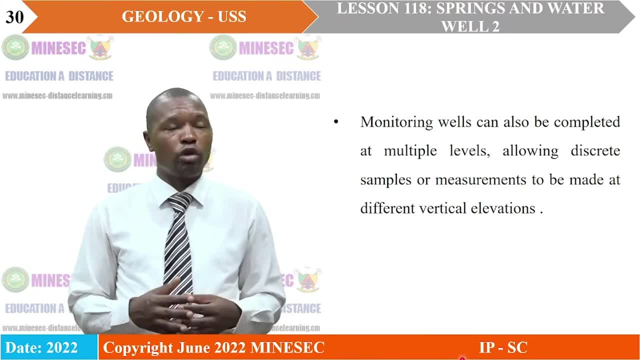 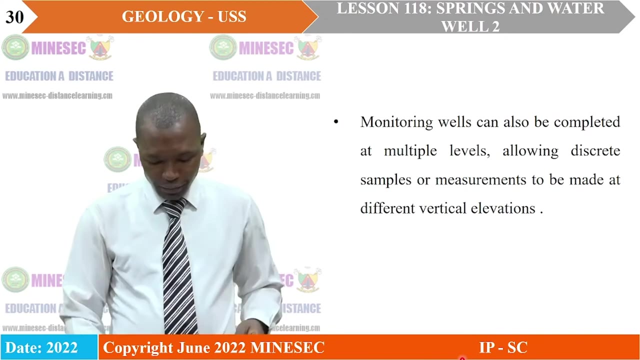 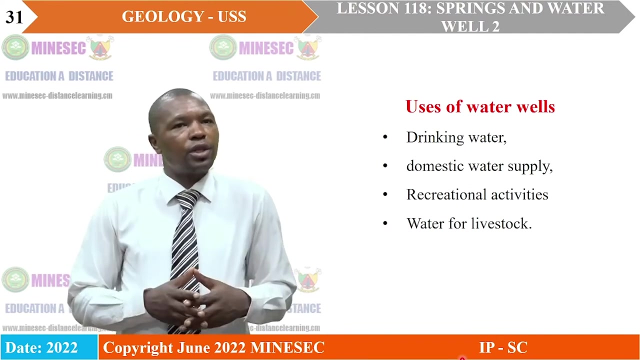 Because these wells are used for monitoring and for scientific purposes, For scientific programs or for research. They could, you know, be docked in different layers as far as the monitoring process progresses. Now, what are the uses of water wells? Water wells are used for drinking. 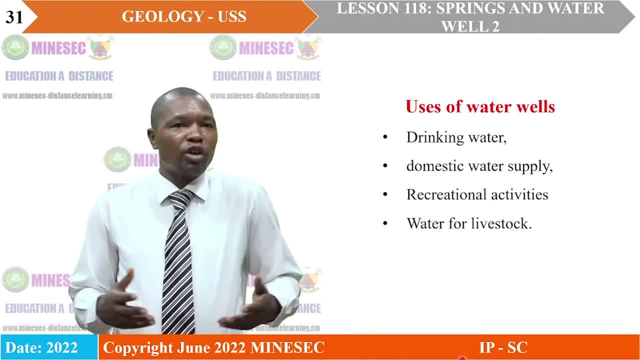 They are used for domestic water supplies And they are used for recreational activities As well as water supply, well as water for livestock. You see that the uses of water wells are related to uses of springs. That is why together, they are generally underground water reservoirs. We 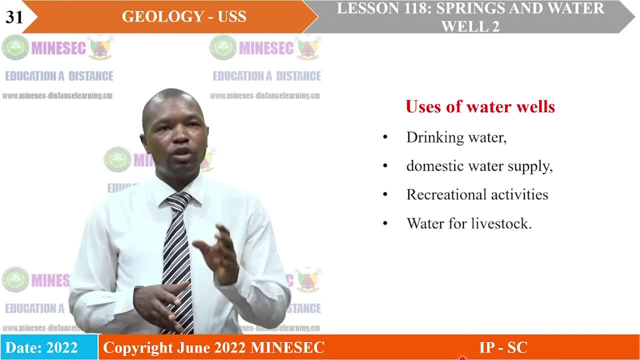 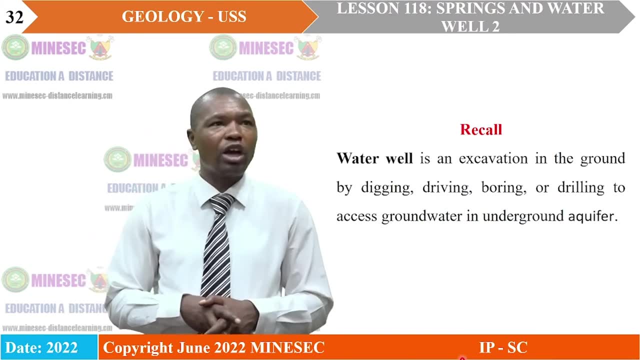 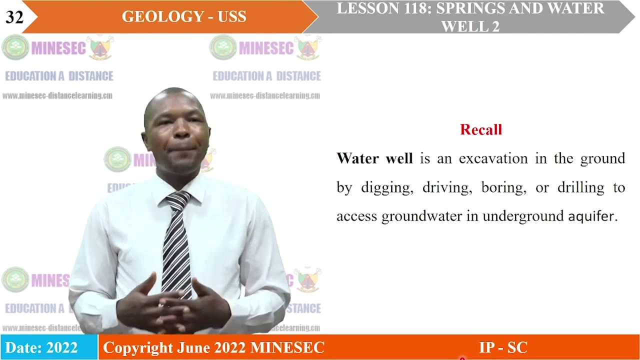 could have a diversity of the uses of wells. Those are a brief caption of the main uses of water wells. Now recall that water well is an excavation in the ground by digging, driving, boring or drilling to access groundwater in underground. aquifer Again that water. 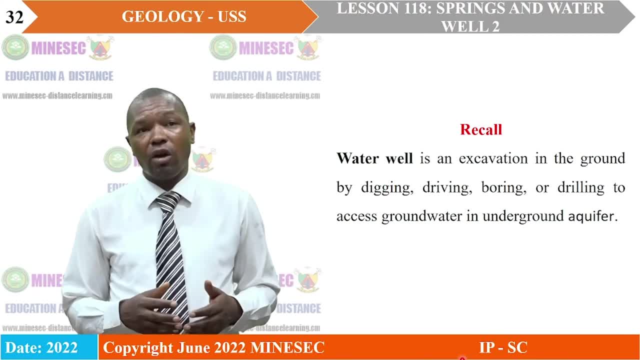 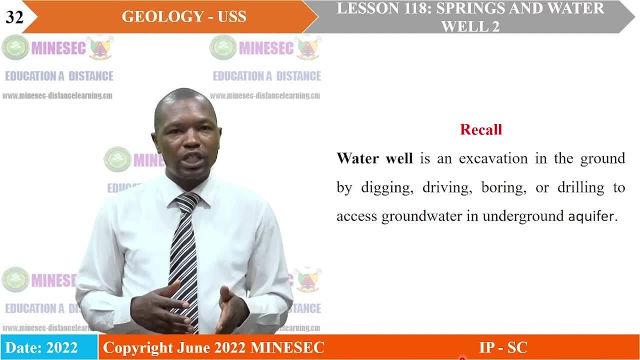 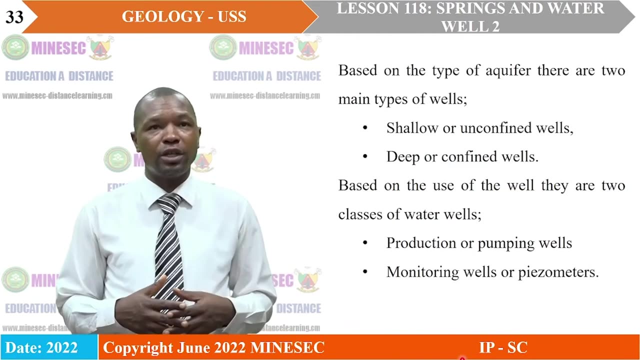 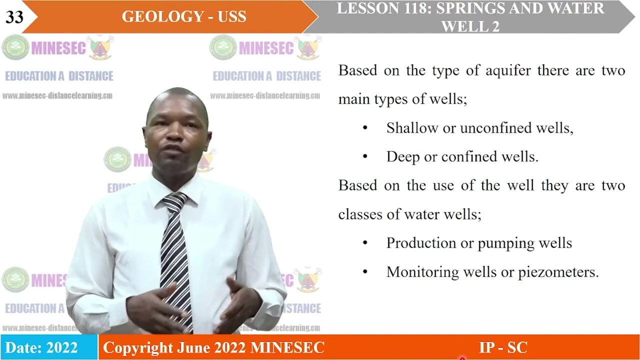 well is an excavation in the ground by digging, driving, boring or drilling to access groundwater in underground aquifer. Based on the type of aquifer, there are two main types of wells. We have shallow or unconfined wells. You have deep or confined wells. Then, based on the use of the wells, 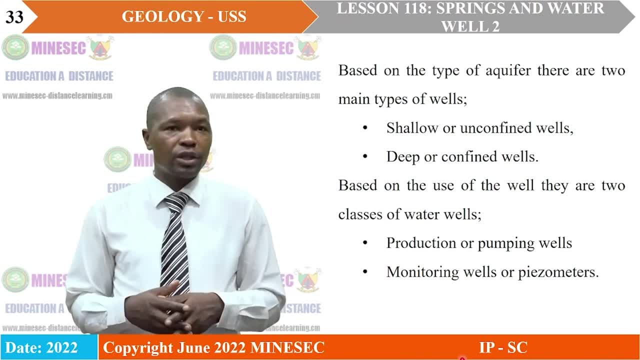 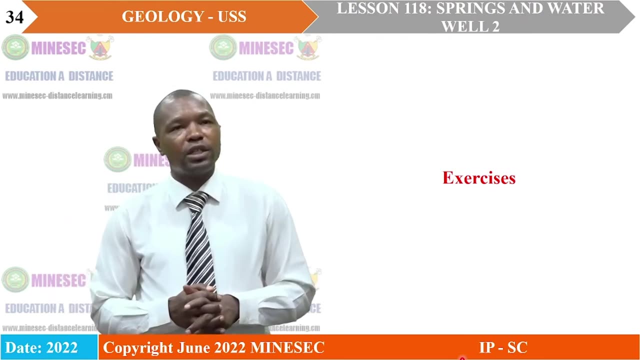 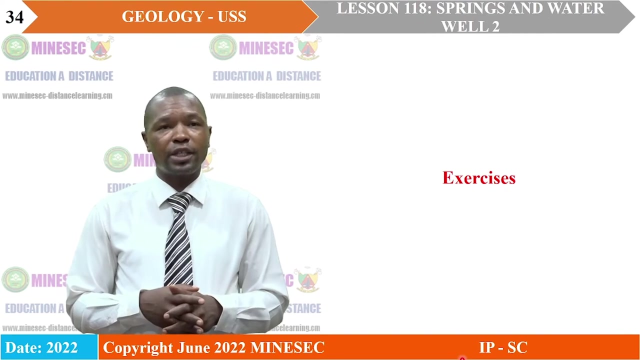 there are two classes of water wells. You have production or pumping wells, Then you have üç hello monitoring wells or caseometers. Have a look at our lesson on water wells, or springs, and water wells too. We shall dive into some application exercises and test. 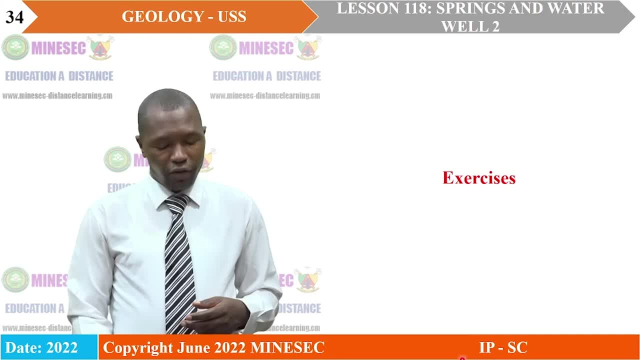 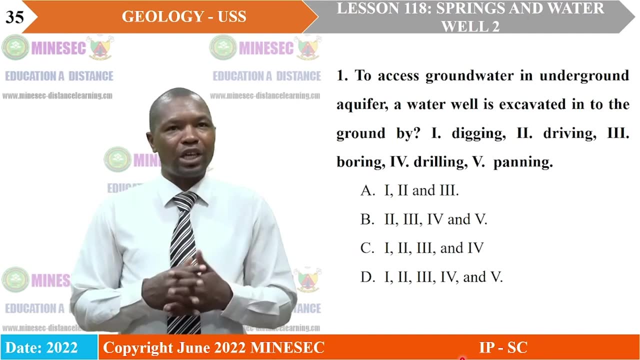 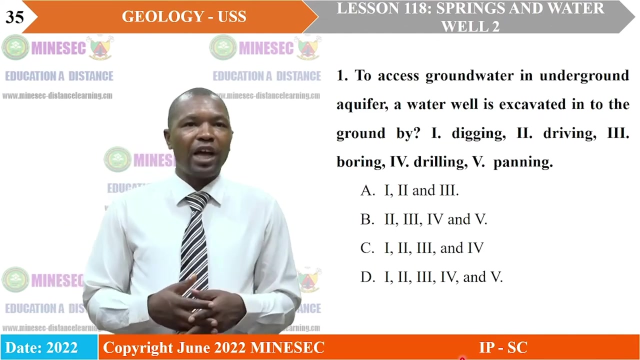 our ability for the knowledge we have acquired in our lesson. Exercise number one: To access groundwater. in underground aquifer, a water well is excavated into the ground by 1 digging, 2 driving, 3 boring, 4 draining, 5 panning- Again our 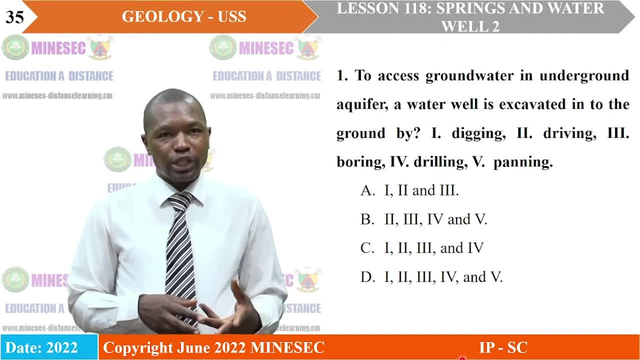 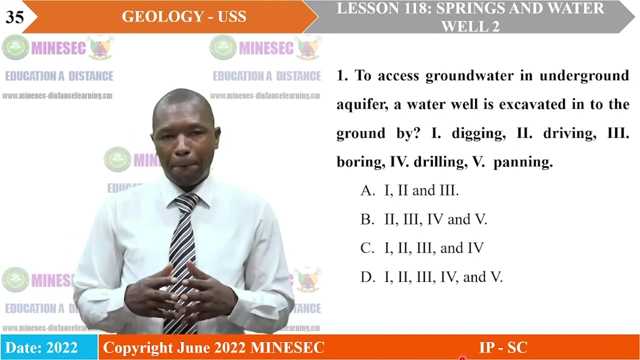 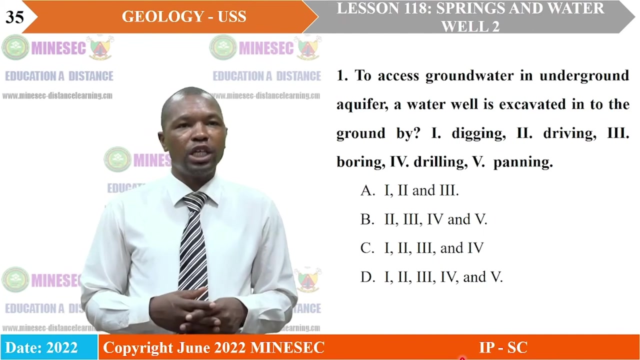 question: To access groundwater in underground aquifer. a water well is excavated into the ground by 1 digging, 2 driving, 3 boring, 4 draining, 5 panning Again. our question: To access groundwater in underground aquifer? a water well is excavated into the ground by 1 digging, 2 driving, 3 boring, 4 draining, 5 panning- Again our. question: To access groundwater in underground aquifer. a water well is excavated into the ground by 1 digging, 2 driving, 3 boring, 4 draining, 5 panning. Again our question: To access groundwater in underground aquifer. a water well is excavated into the ground by 1 digging, 2 driving, 3 boring, 4 draining, 5 panning. Again our question To.